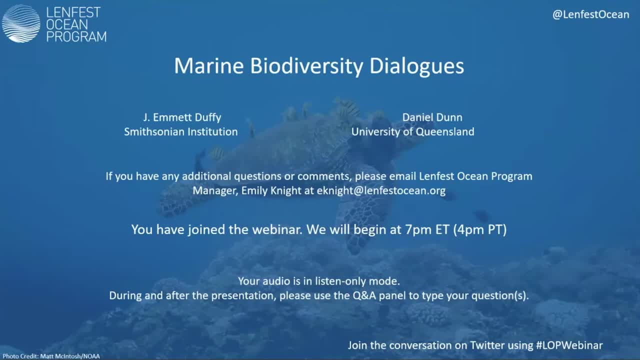 but we wanted to highlight in the title that the outputs of this project, which will be a spatial gap analysis and a framework by which we can assess marine habitat and biodiversity, will come from just that: dialogue, Dialogue across two expert working groups, the first of 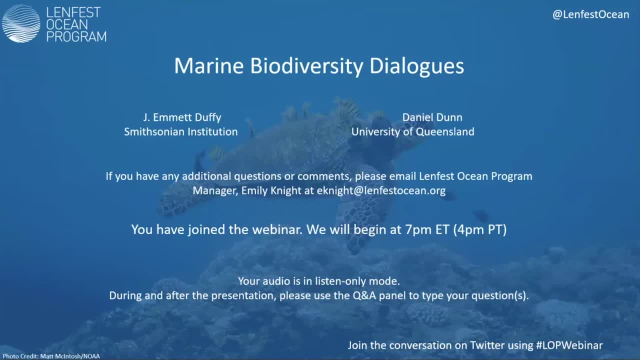 which recently started, And through their collaboration, those working groups will wrestle with concepts related to measuring and monitoring marine biodiversity, including discussing case studies from across the world. We'll also have an introduction from Chris Zari, President and CEO of the National Marine Sanctuary Foundation. The Sanctuary Foundation is our partner in supporting 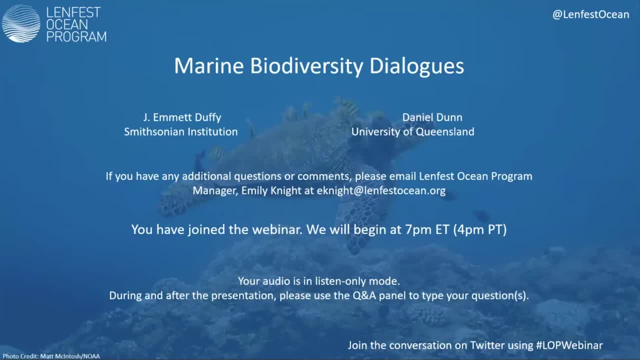 this project, and Chris is very much at the forefront of why this project is so necessary. So, finally, this webinar is what we at LENFest like to call a launch webinar, That is, a webinar that we provide at the beginning of the project. 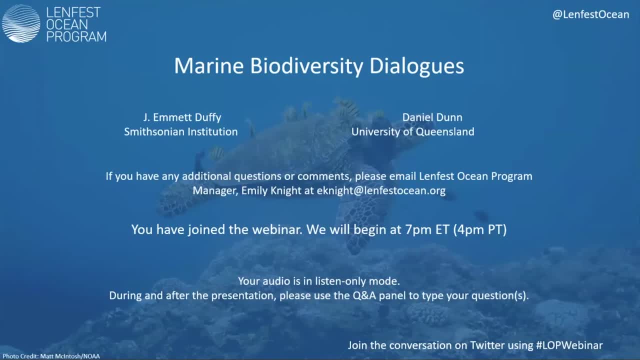 Thank you, Emmett, and thanks for that entry Sell. what would you like to see at the beginning or a start of the webinar? So this webinar is about how to center or structure an education initiative. So in this webinar series we are going to be focusing on how to be a more inclusive citizen. 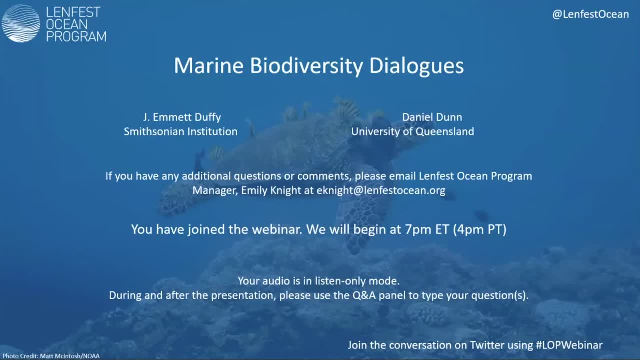 of a species and to have people engaging in the Community. So some of you have probably heard about this training program, OECD, And so OECD is a set of VNESA or OECD Agricultural Institution, or SEAS, that supports the development of a community based education and services. The project is designed to support and support social 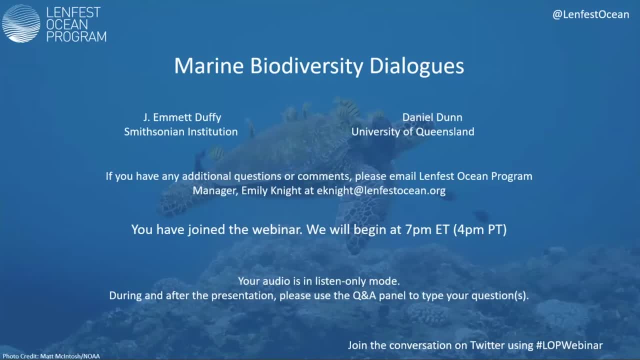 environmental and cultural events that are important to all Chamber members and community members, And as we are focusing on the work that OECD is doing and our goal being to promote transparency and engage audiences from the outset of the project or unsure, if you are, just send me a note. My email is on the slide. I'm pretty easy to find. 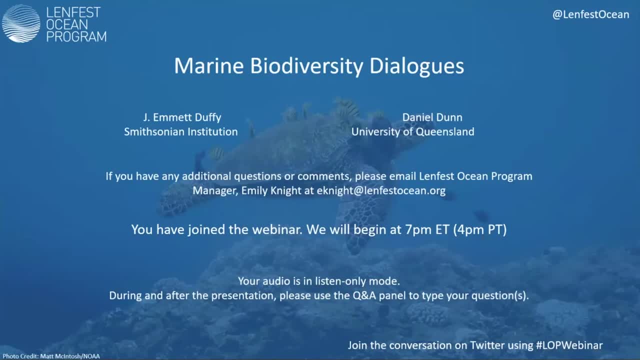 Second, we are recording this webinar and we will distribute the link broadly and hope you will forward it to your networks. A few webinar logistics. We have all attendees muted with so many people on the line. This is just to prevent feedback or echoes. We will have time for the end. 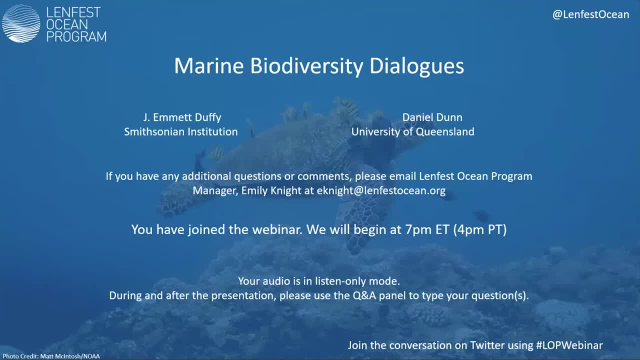 for questions. Use the Q&A panel to type and submit your question at any point during the webinar today. We'll keep track of the queue and I will read the question aloud at the end for the researchers to answer. And if you type it into the chat, that's okay. I will do my best to follow that. 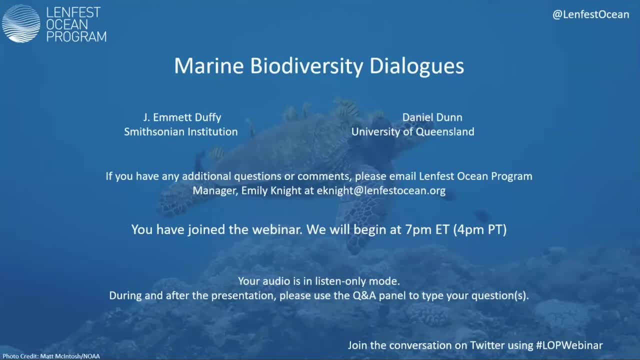 as well. But we will keep track of the queue and I will read the question aloud at the end for the researchers to answer. But we prefer kind of keeping it all in one place in the Q&A panel. Also, we might run out of time for questions If you submit a question that doesn't end up. 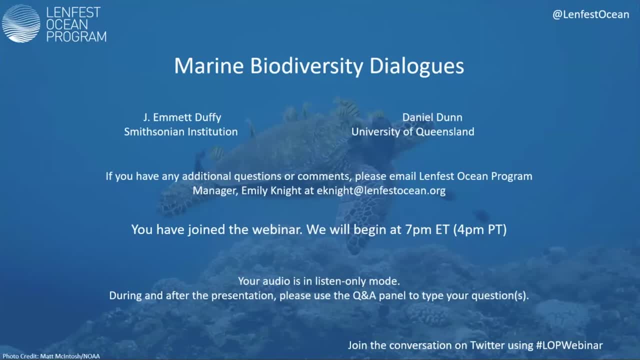 getting asked. we do download all of them so we will see your question and can always follow up. And we also welcome you to follow up with us either at LenFest or the researchers. So at this point I am going to turn the mic over to Chris. 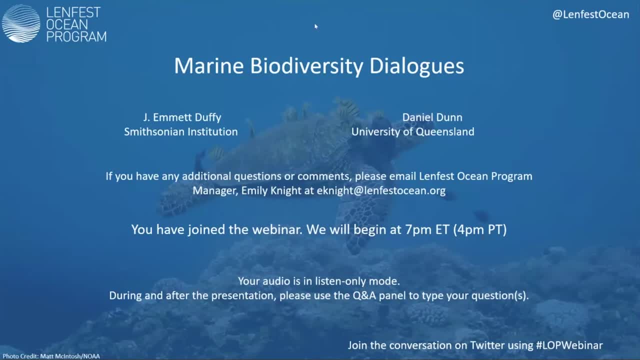 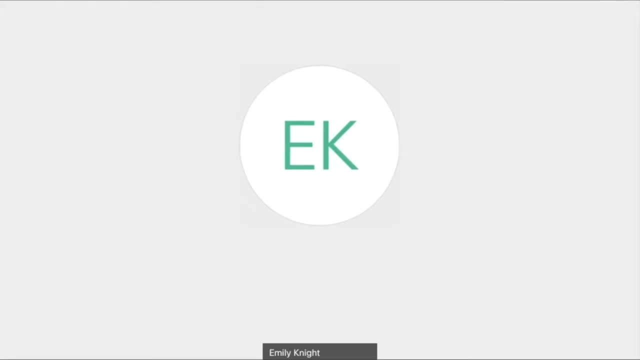 Chris, who's going to give an introduction to this project. Thank you, Emily. Thank you, Thank you for everyone who's joining us this evening. My name is Chris Seri, President and CEO of the National Marine Sanctuary Foundation, And I want to also thank the LenFest Ocean Program for working with us on this project, and also the 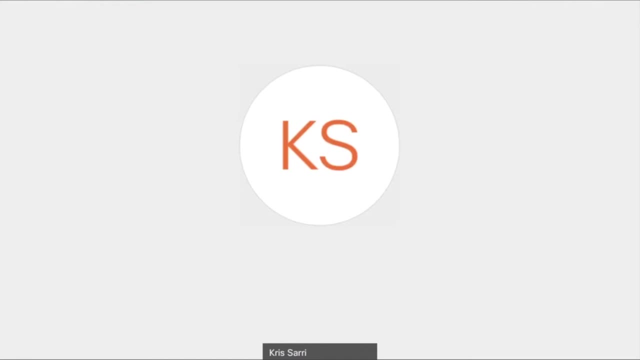 Gordon and Betty Moore Foundation for their support for this effort, And so, for those of you who don't know, the National Marine Sanctuary Foundation. we're a nonprofit organization and we work very closely with NOAA to increase stewardship of our oceans and great lakes. 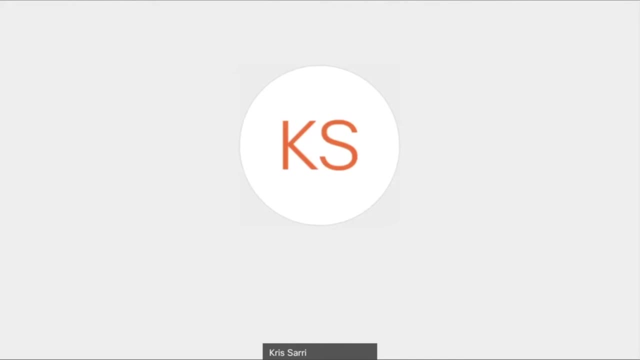 And one of the important ways that we do this is we try to increase awareness and support for our central network of protected waters and national marine sanctuaries and marine national monuments- The Russian. The rationale behind this, this project, is pretty simple. You know, as humans, we depend on a healthy planet for our livelihood. 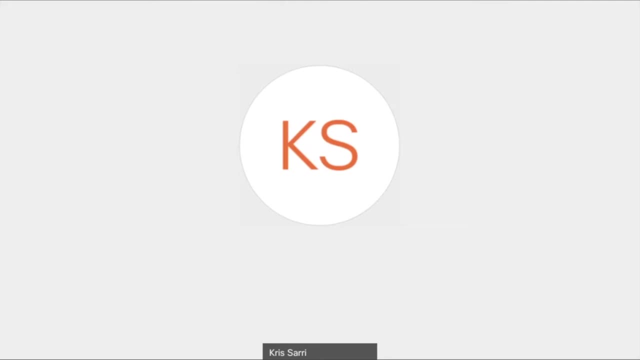 And a healthy planet depends on a healthy ocean, And a healthy ocean depends upon the variety of life that's supported in it and the habitats that it can maintain, And, as we know, we're losing species diversity, with harmful consequences for both the environment and humans. 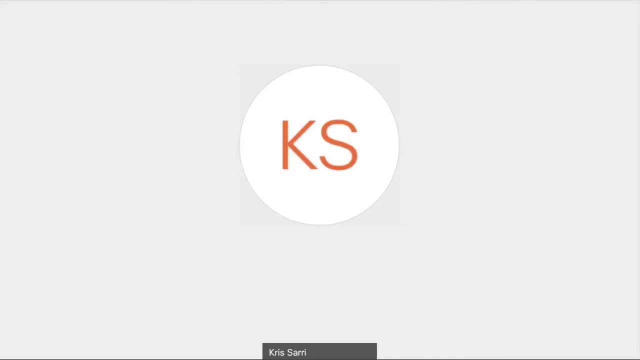 And so we wanted to work on undertaking this project with the question of: if you wanna have a healthy ocean, what are those key areas that we need to protect for marine biodiversity, And so the idea came to develop a framework that assesses where there's gaps in, and to what extent, marine protected areas in the US. 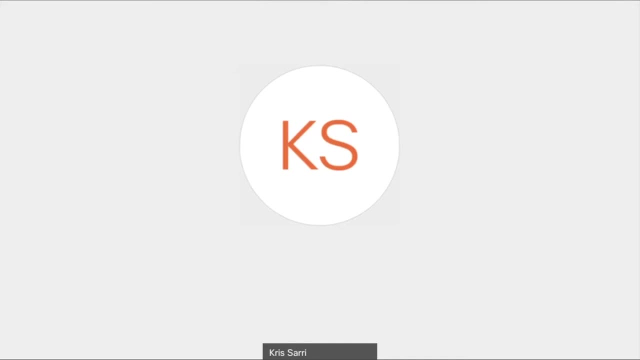 are helping to protect biodiversity from the nearshore to the borders of the US EEZ, And the idea of this framework is: ultimately, it becomes a tool that decision makers, natural resource managers and stakeholders can use at local, regional and national levels. 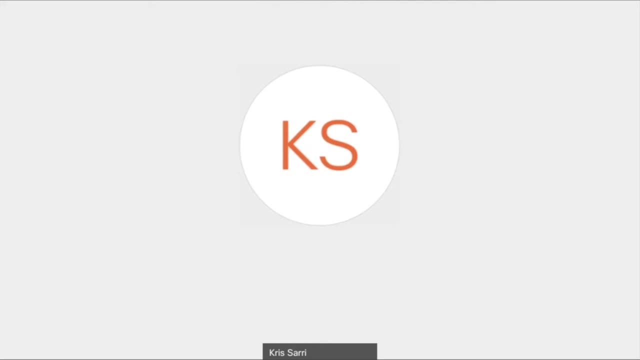 to determine what types and percentages and approaches that we need to take to managing ecosystems, And this is really important as we talk about wanting to protect 30% of nature by 2030.. Where we put these areas, the level of protections all have a tremendous difference. 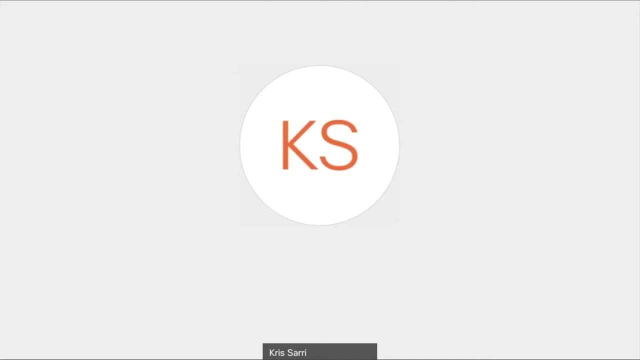 in terms of the health of our ocean. So the work that Daniel and Emmet will discuss tonight actually kind of arose almost 20 years ago from an executive order that called on us to do a scientifically based, comprehensive national system of MPAs that would represent diverse US ecosystems. 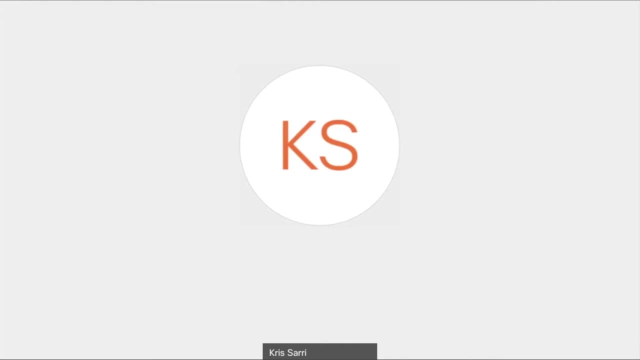 And 20 years later, we actually haven't been able to do that, And this is really a start of that effort to look at what is a comprehensive national system of MPAs that represent diverse ecosystems And, as we know right now, that we have gaps in representation. 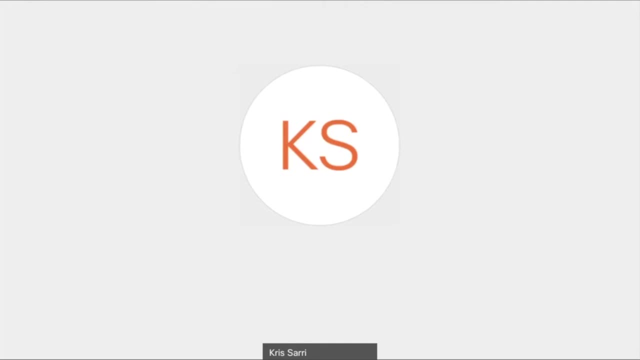 we have ecological gaps and we have management gaps, And so understanding from a science framework about how we can address these gaps from a management and policy perspective is very critical, especially to national marine sanctuaries and marine national monuments. how do we actually make sure as we look to expand the system and designate new sites? 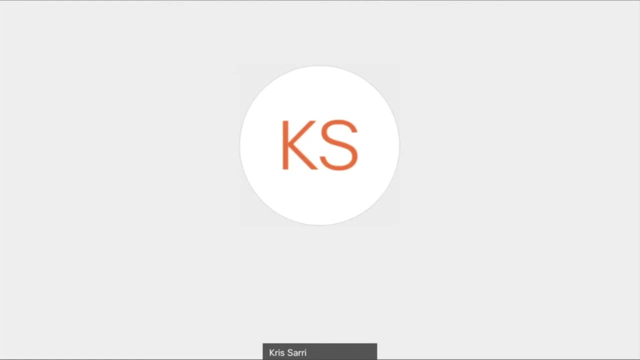 that we're really looking at those opportunities that will help increase our biodiversity. So I'm very excited that this is the start of a process where we can look at the scientific and face comprehensive way to look at how do we protect biodiversity in our oceans and 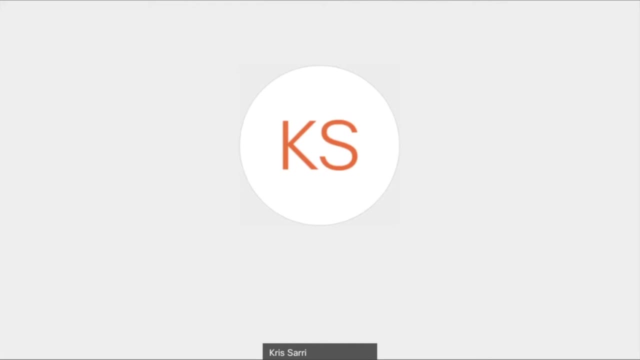 really look at it from both the health of the ocean and also the role that it helps play in terms of the health of human communities too. So thank you, Emily, and I'll turn it over to Emmet and Daniel. Great, thank you so much, Chris and Emmet, do you want to? 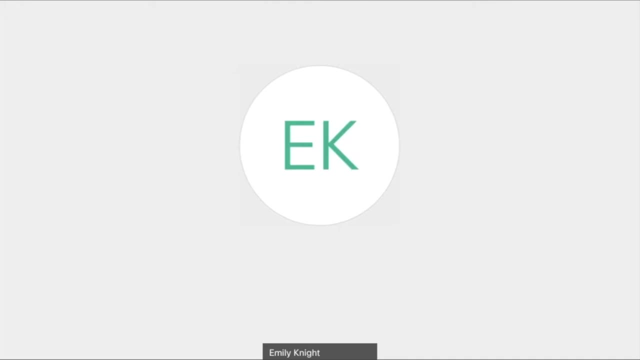 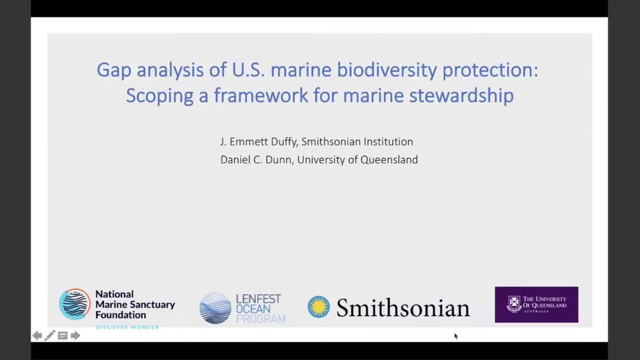 launch into the presentation about the project Sure, Yes, hi, everyone. let me share my screen here and I'll be right with you. So welcome to everyone. it's a pleasure to be here and to share our plan for this important project. Can you see my, my slide? 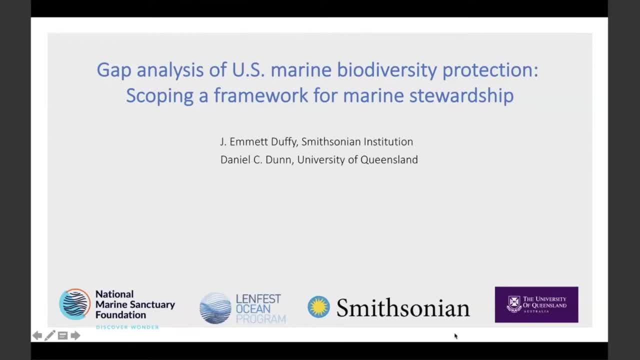 Just checking. so this is a project that that Daniel and I- and I hope everyone involved- hopes will provide a foundation for a renewed, data-rich approach to marine biodiversity protection, and I'd like to thank the Lenfest Ocean Program and the National Marine Sanctuaries Foundation for supporting this. 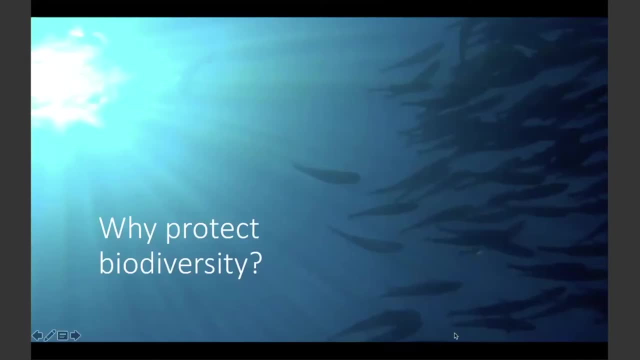 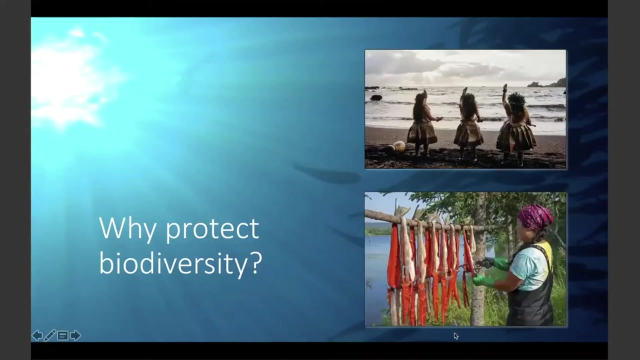 work. So I'd like to begin with the basic question of why we should be protecting biodiversity in the first place, and there are, of course, many reasons for this and many answers that could be given. Nature provides inspiration that can't be valued, but also utilitarian services- fisheries, aquaculture, coastal protection and so on- and diversity. 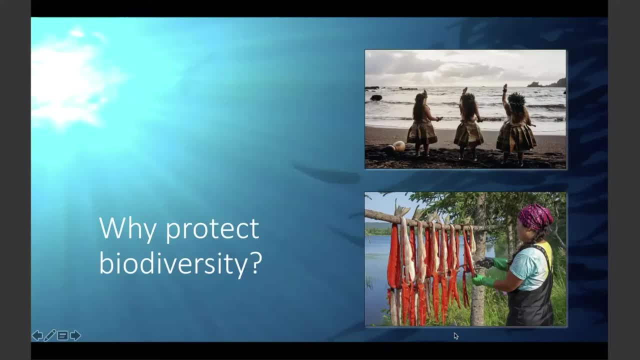 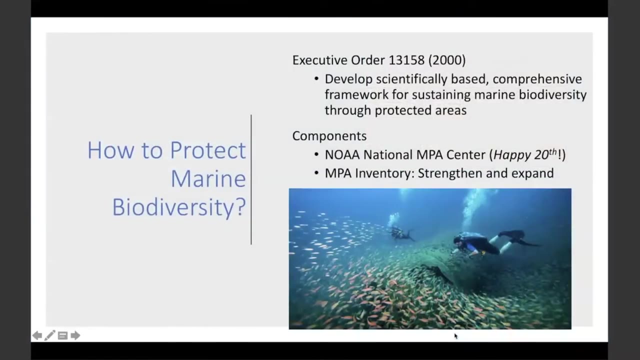 strengthens ecosystems. but despite these benefits, biodiversity is is really threatened in in many areas around the world by over harvesting and coastal development and pollution, among among other threats. So the question is: how do we protect biodiversity in a way that is sustainable into the future but that is also compatible with the human uses that that we have? 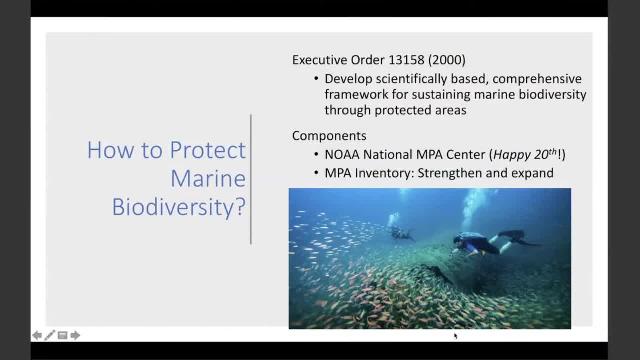 for the ocean, And Chris mentioned that that much of this began with- or I should say was- was formalized with President Clinton's executive order in 2000, which was meant to to develop a scientifically based framework for for sustaining biodiversity in protected areas, And that led to. 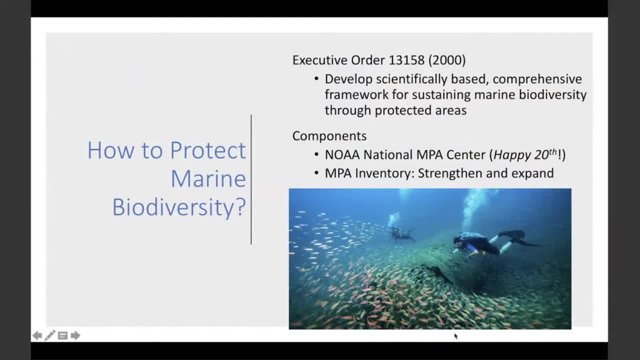 the development of the NOAA's National MPA Center, which is celebrating its 20th birthday this year, and to the MPA inventory, among among other things, which is charged with strengthening and expanding the, the protected area network, and and partnering with others as well. So in 2015, 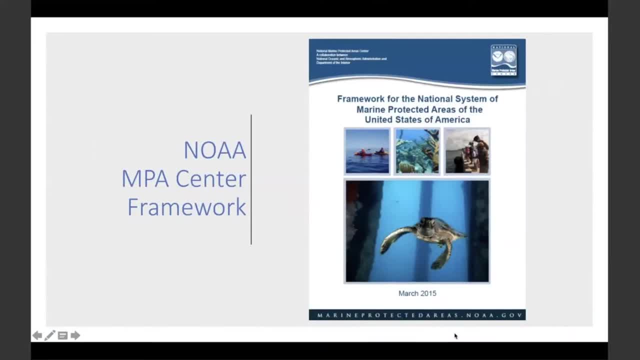 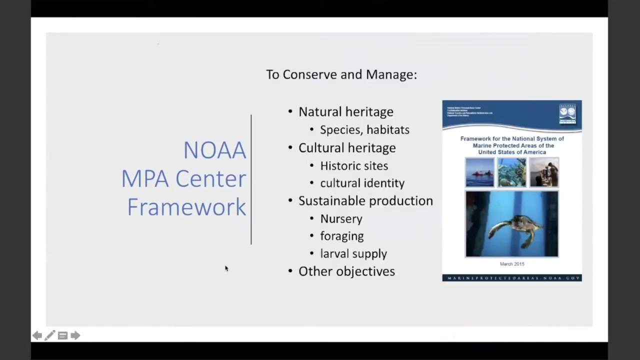 the, the MPA Center, produced this framework and see if I can move this. yeah, Okay, produce this framework for the protected areas and and included several, several goals for the for the United States network. These include protecting or conserving and managing natural heritage, what we think of as biodiversity, species, habitats, the processes that happen in them. 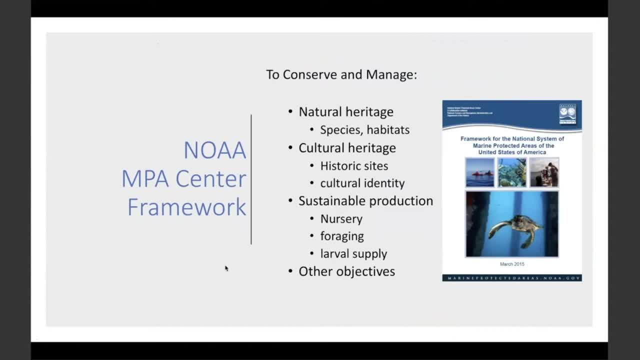 as well as cultural heritage, that is, that is important to humans, and this involves historical sites as well as important areas for cultural identity. And then finally, of course, to to ensure sustainable production of fishes and other resources that people use from the ocean, by producing nursery for protecting nurseries and foraging areas and multiple supply, and so on. 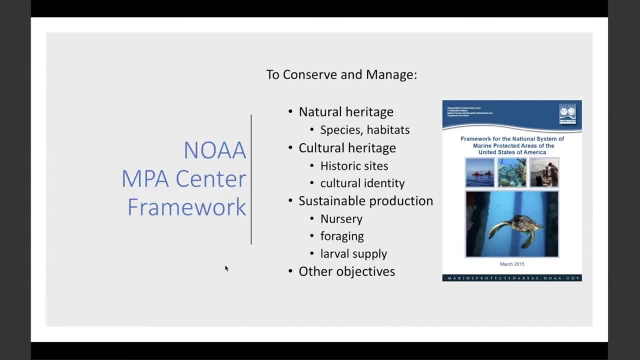 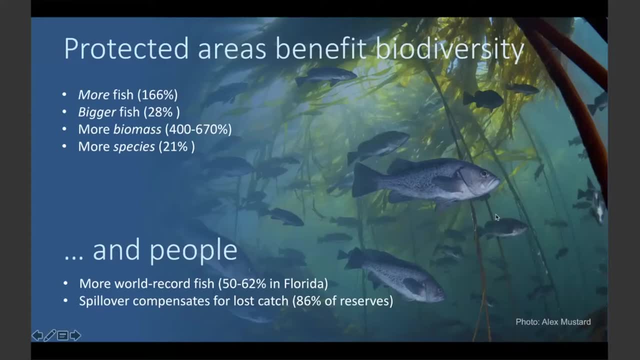 And there were other objectives as well. So there are a number of reasons, or a number. there's now considerable evidence that protected areas benefit biodiversity from from several perspectives. I'm thinking about it from from the fisheries perspective. protected areas generally have more fish, bigger fish, more biomass and also more species, particularly if they're if they're. 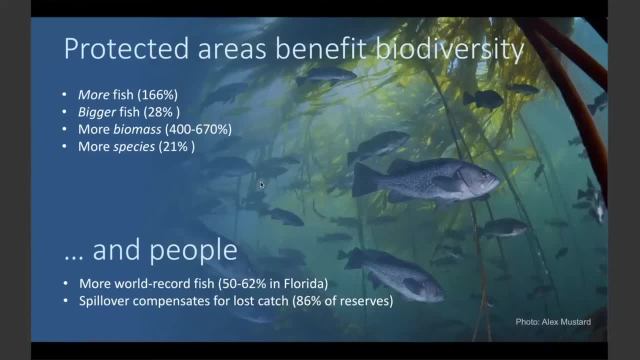 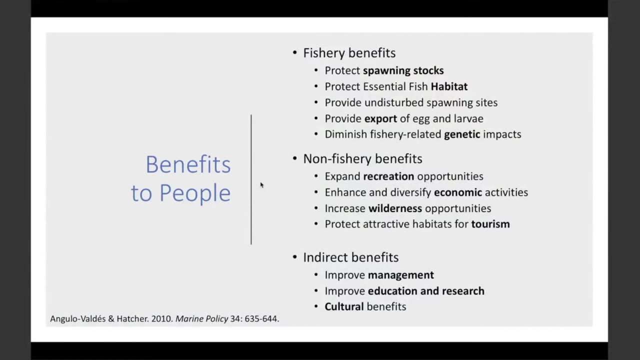 well, well enforced, but also have benefits for people in terms of spillover of fish to outside areas as well. So these- these have been documented well elsewhere and we won't spend much time on them, except to say that, in addition to these fisheries benefits, there are also benefits in: 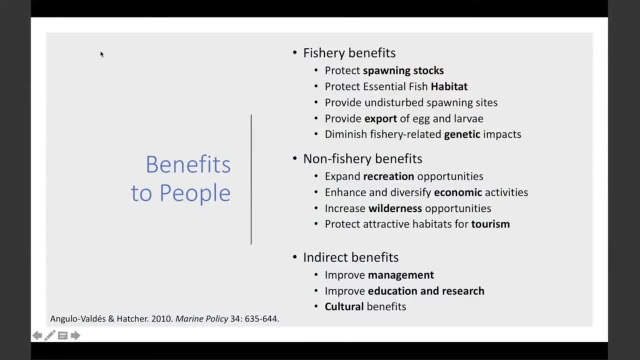 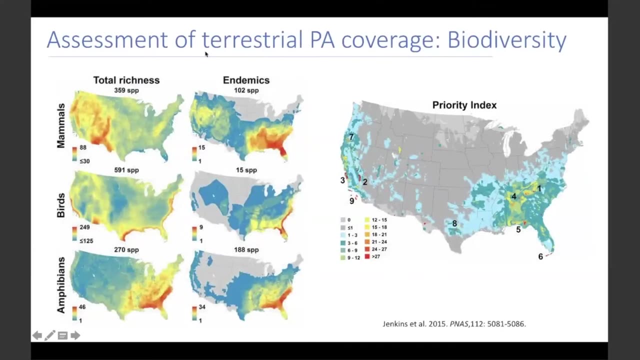 many other ways, including recreational opportunities, attractive habitats for tourism, and so on. So this brings us to the question of how to make sure we are protecting what we need, given that there are multiple uses of of land and sea. And so in in the marine realm, in the ocean, answering. 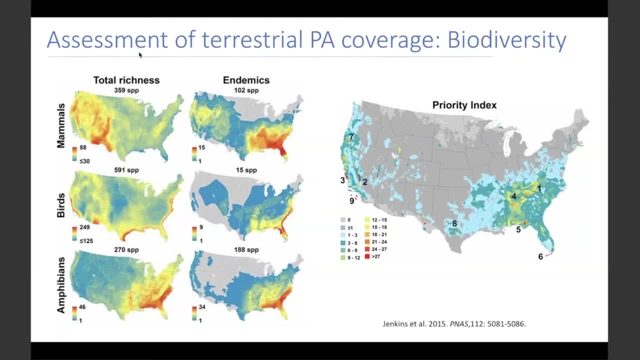 this question is really at a pretty early state, and so we can turn to the experience on land, to ask to, to, to look for lessons learned on the uses of land and sea, And so I'm going to turn it over to Dr learned on how to optimize protection of biodiversity within the country. 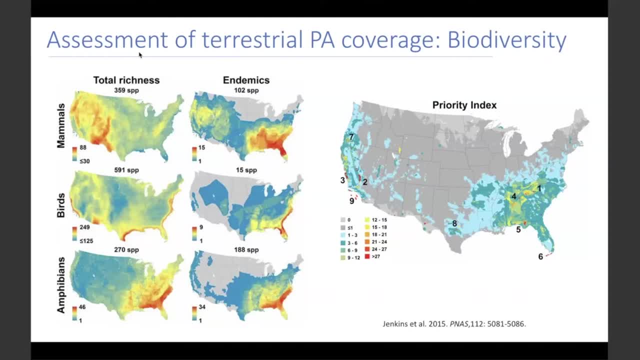 And so there are good data on both biodiversity and protection on land, and we have looked at this from a couple of different perspectives. One is to ask where the biodiversity is, and there are various ways of looking at this, including the species richness, that is, the number of species, of particular kinds of animals. 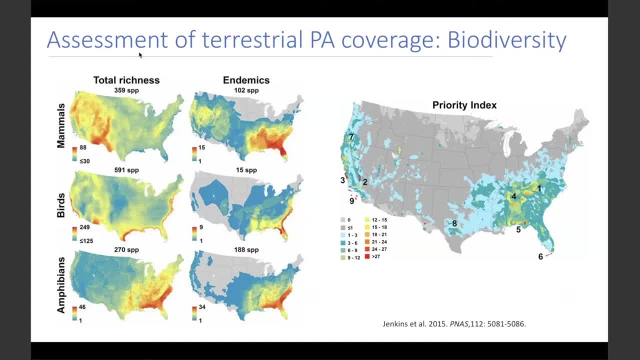 and plants, but also the degree to which they are unique and live only there, the number of endemics- And as you can see, that varies a bit among different groups- And then, when that is overlaid on the areas that are protected, the prioritization results. 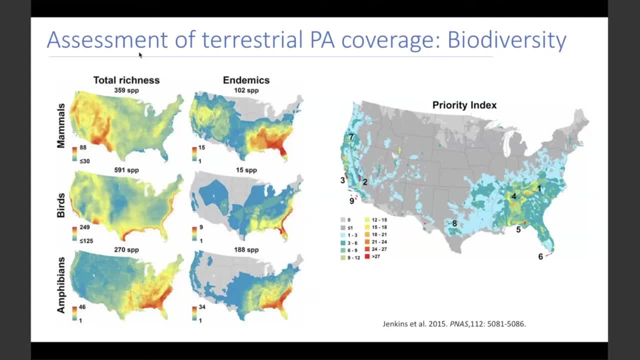 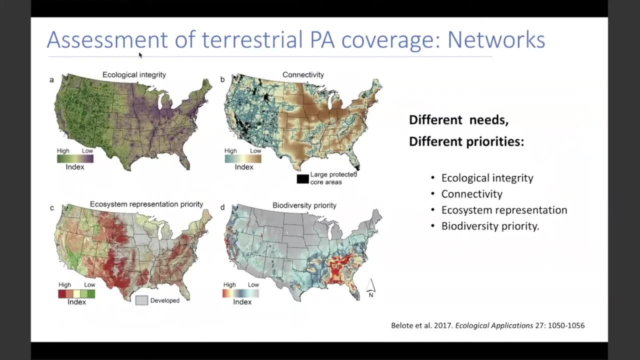 in selecting places that are high on the score of having richness. So this is one way to prioritize protection, or one of the criteria, But we also have to consider how all of those different protected sites might work together in a network, and this is because, particularly in the warming world in which we find ourselves, 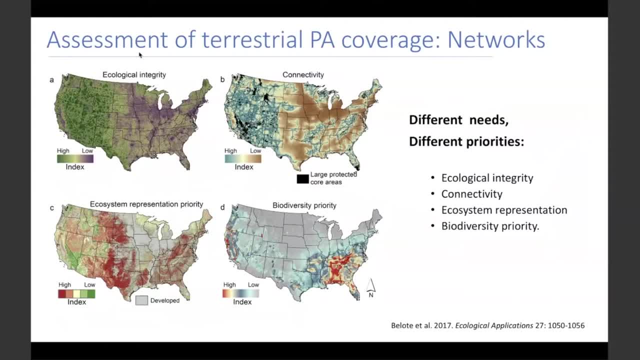 now. organisms move around and we need to be able to sustain them, those populations, for future generations, And that requires designing the networks in such a way that the organisms will be able to move. So that's the principle of connectivity. There is also the criterion of ecosystem representation. 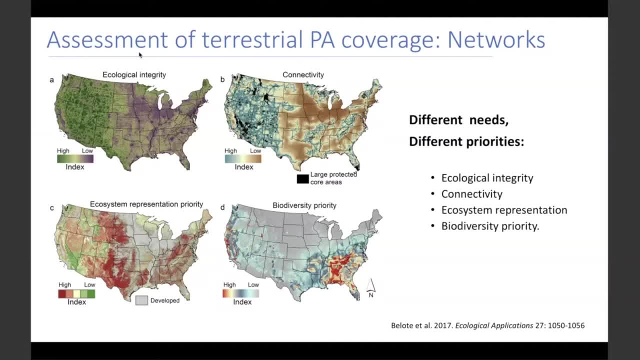 That is, we're interested not only in isolated species, but also in the kinds of ecosystems that they live in, And so ecosystem representation- such as in the lower left corner The map here- is a criterion as well, And again, these are different needs. 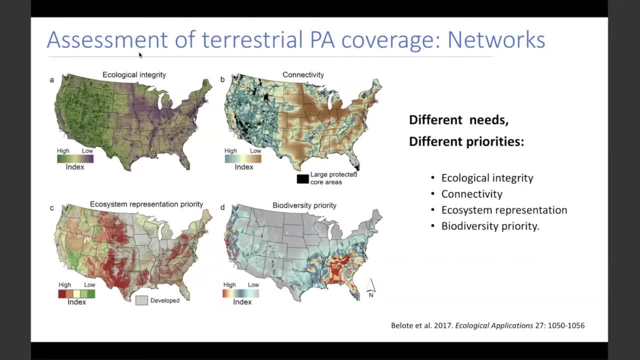 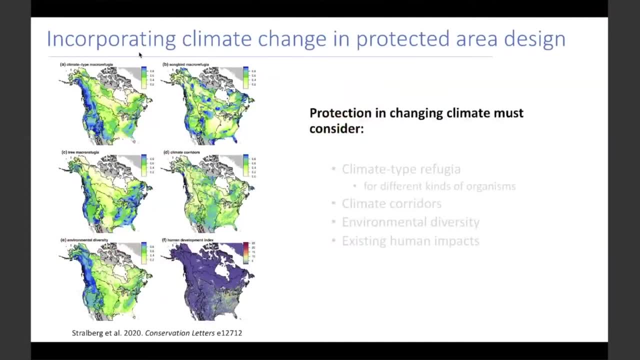 They need to be balanced to prioritize conservation. This is relatively well done on land, but still poorly known in the ocean. And finally, as I mentioned, for connectivity, an important aspect is preparing for climate change, And so that entails considering aspects of the landscape. 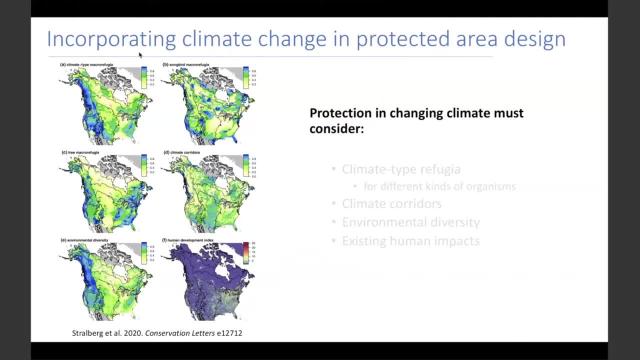 And so that's the first thing that we need to consider, And then, finally, as I mentioned, for connectivity, an important aspect is preparing for climate change. We need to consider the landscape and land forms that allow organisms to have refuges or refugia from changing climate, and also climate corridors that allow them to move. 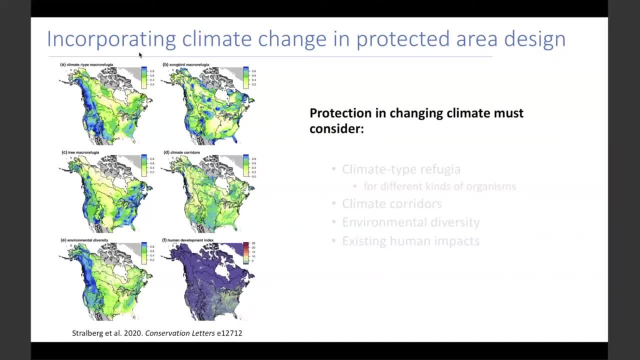 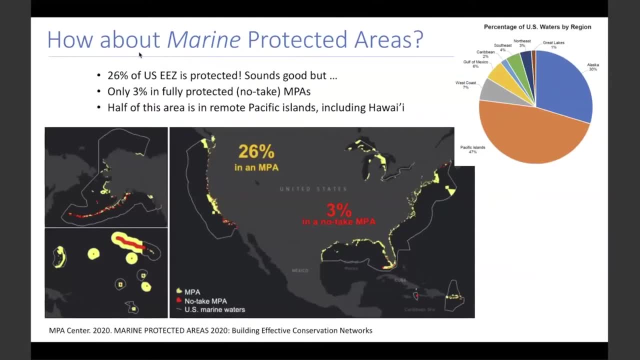 as the climate warms. So this has been done on land and is only beginning in the ocean. So that brings us to the question, After having looked at some of the experiences From terrestrial systems, of how our marine protected areas are doing or how we're doing. 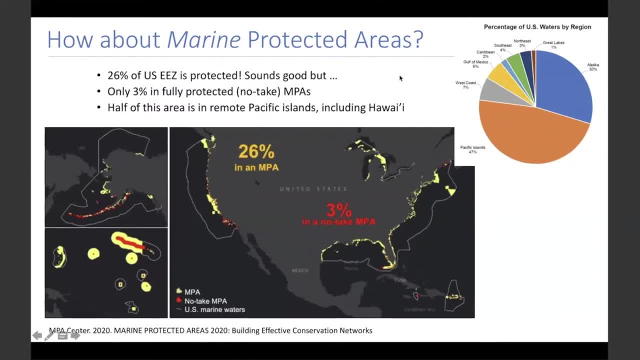 in protecting biodiversity in the ocean. I should first emphasize that the United States has nearly 1000 marine protected areas of one sort or another across our many regions and in fact 26% of the US exclusive economic zone is under some form of protection. 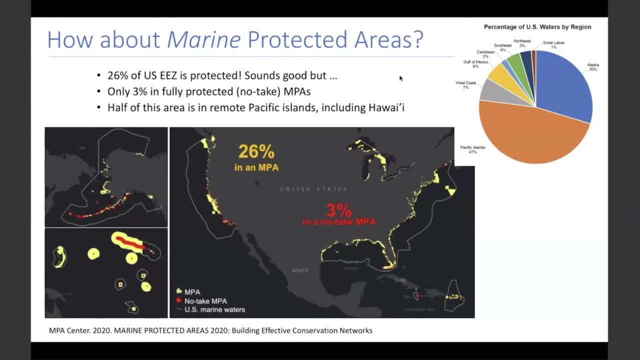 Which sounds great, But it's also true that only 3% of that is in fully protected or no-take MPAs, which science shows are really the best way to protect and sustain biodiversity. And finally, of that protected area, almost half of it is in the remote Pacific Islands, including Hawaii. 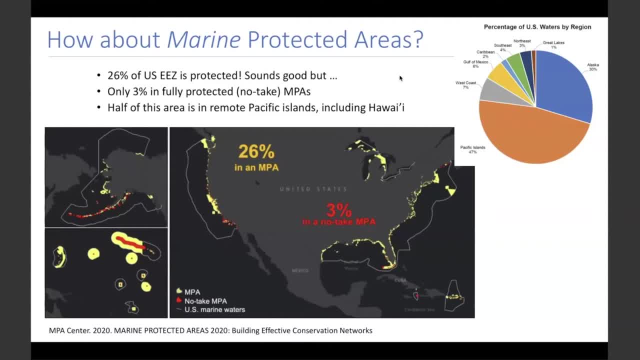 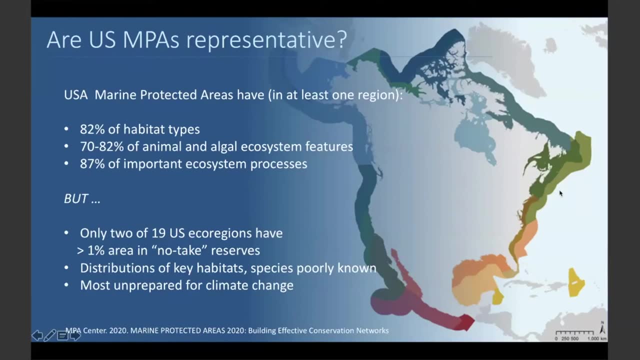 So there is a fair amount of work to do in reaching the goals of 30% in the coming decade or so. So, in addition to the total amount of area protected, the question also becomes: how representative are these protected areas in the United States? 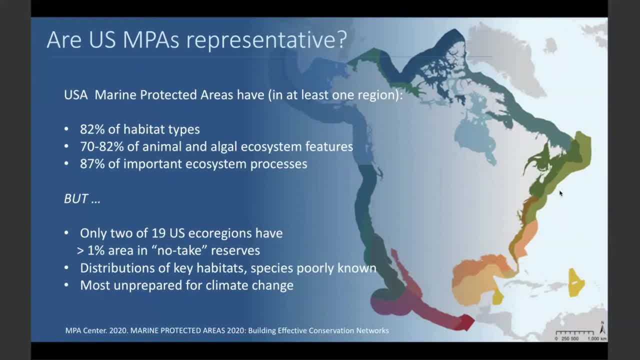 And so the good news is is that, across the network of protected areas in the US, 82% of the marine habitat types that are recognized are represented in at least one of the 19 ecoregions in the United States, And somewhere between 70 to 80% of major animal and algal or seaweed ecosystem features are also protected. 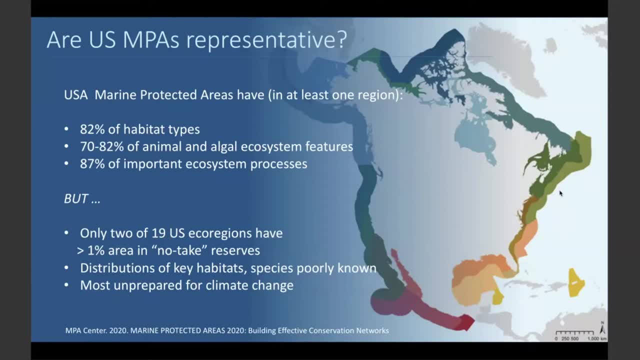 And many of the processes. Again, though, it's important to point out that many of these are sort of one-off instances, And there are really only two of the 19 US ecoregions- coastal ecoregions- that have more than 1% of their area in no-take reserves. 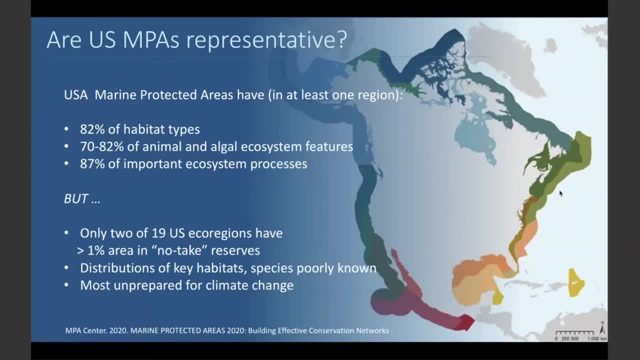 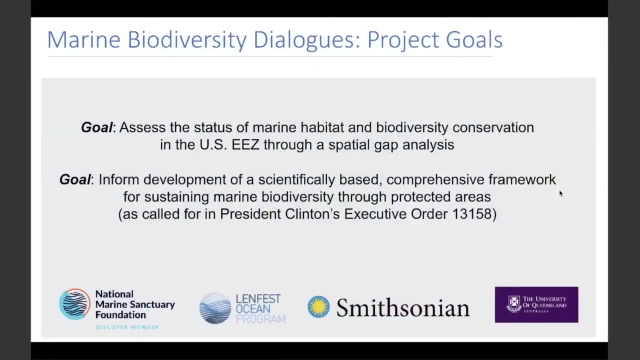 And it's also true that the key habitats in many of the species of marine animals in our waters, their distributions, are poorly known. And finally, as I mentioned, we're really not prepared for climate change as these organisms start to move. So this was part of the rationale for why we need a spatial gap analysis of marine biodiversity. 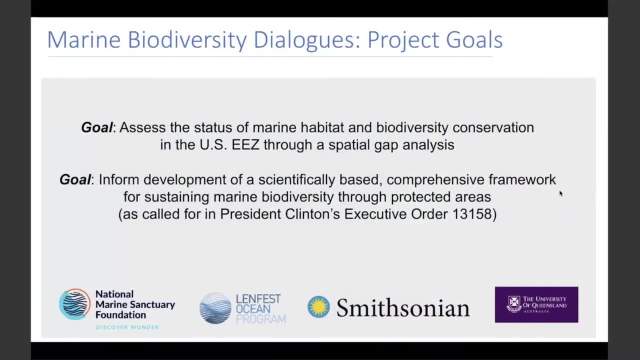 So that brings us to the current project, the Marine Biodiversity Dialogues, And our goal simply is to assess the status of marine biodiversity- both habitats and species- and conservation within the US EEZ through a spatial gap analysis. Again, this goes back to the executive order's charge of developing a scientifically-based, comprehensive framework. 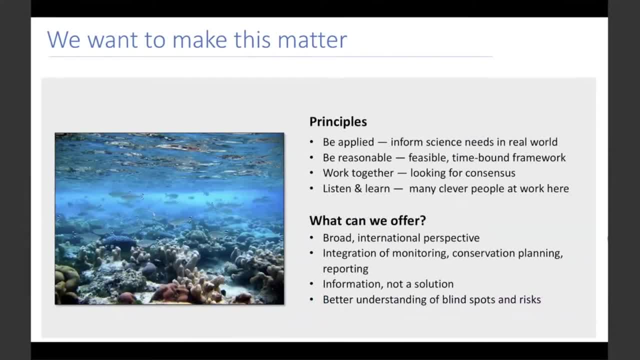 And it's really important to point out that we are keen to make sure that the results of this analysis matter. That is, we want to… We want what we find out, the science, to be applied, that is, to inform conservation in the real world. 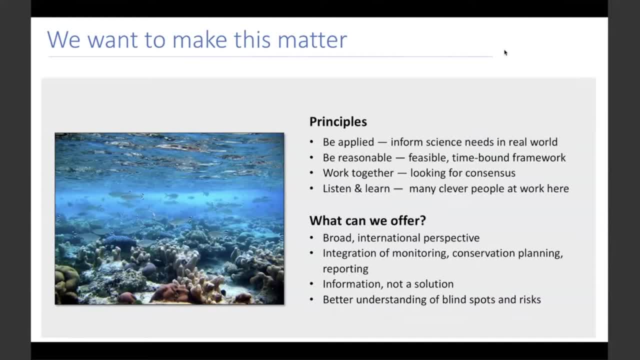 to be feasible and possible within a time-bound framework, working together. So we are looking for consensus and to listen and learn, And to do that we have convened a very diverse and smart group of people, which we will mention in a few moments. 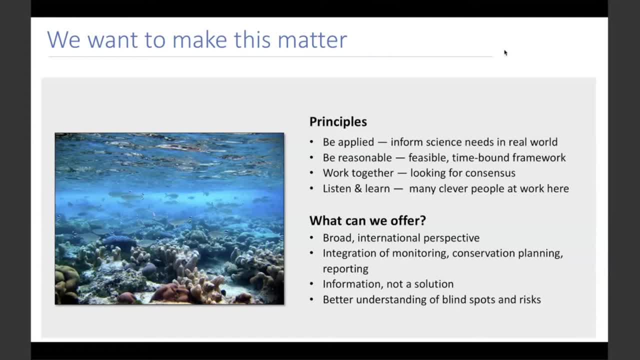 to come to that and to synthesize what has been learned. So what can this project offer that perhaps hasn't been done before? The first is that we have… We're bringing a broad international perspective, looking at what has worked in other places, what hasn't worked. 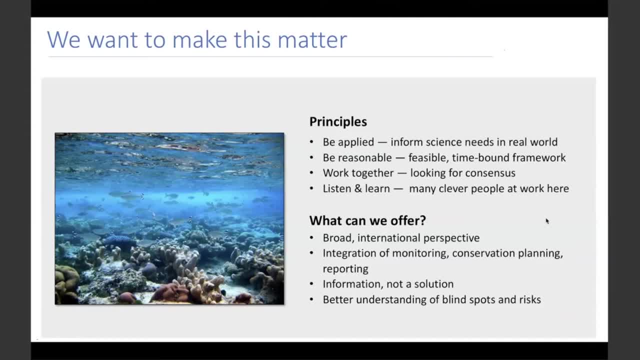 And we also are importantly integrating the biodiversity monitoring perspective that has developed extensively in recent years with the conservation planning framework that is used in many national regional conservation plans. Finally, it's important to point out that the Marine Biodiversity Dialogues project is primarily about providing the information that will allow an informed solution. 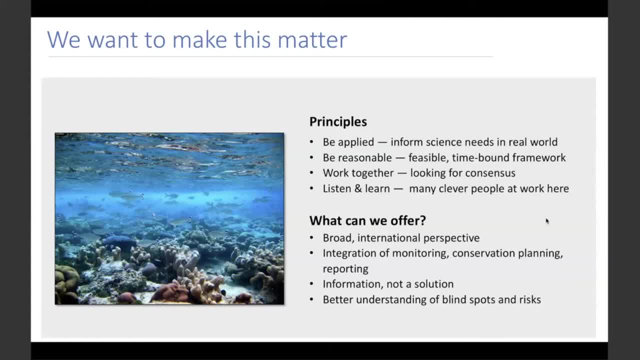 and informed conservation plans to be made. We are not offering a solution ourselves, but the best information that we hope can inform that. And then finally, over the course of this time, we hope that this will give us a better understanding of some of the risks and pitfalls that we might find on the way. 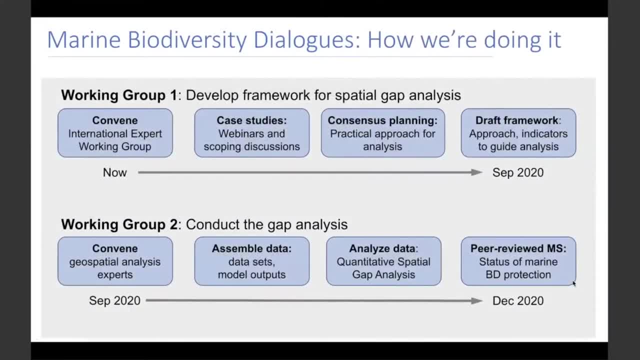 So this is a roadmap, as it were, of where we're going, And the project is proceeding in two phases: The first and both of these have working groups of experts with broad expertise. The first is to develop a framework for the spatial gap analysis. 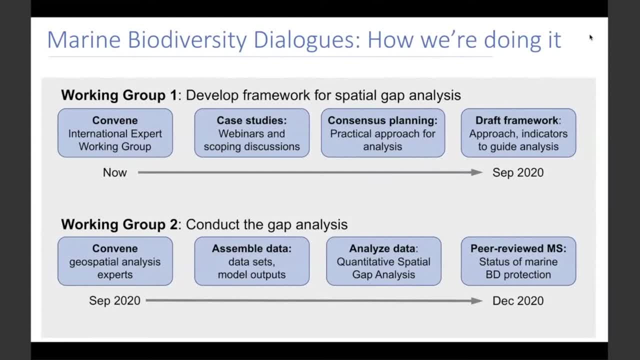 And what I mean by that is to think carefully about the kinds of approaches that are going to be needed, the types of biodiversity that are going to be needed, the types of biodiversity that are most important and most indicative of the health of the ecosystems on which to concentrate. 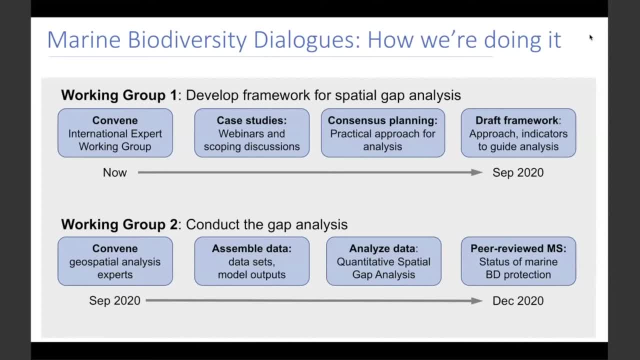 And then to synthesize that into recommendations for how we then go forward with the second phase, which is the quantitative gap analysis itself, And that phase will take the draft framework that was produced by the first group and really bring the geospatial analysis. 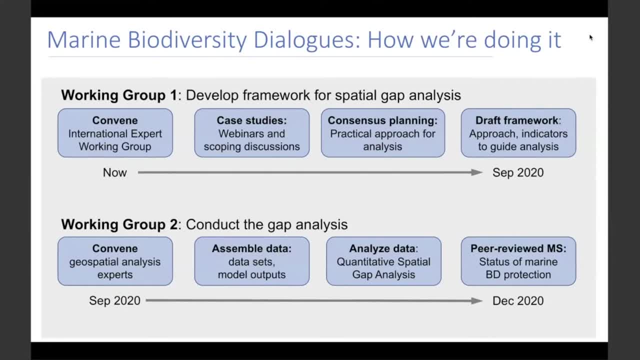 experts together to assemble available data, analyze that data in a spatially explicit framework and then develop that into a peer-reviewed manuscript- one or more manuscripts that are able to quantify the status of marine biodiversity protection in US waters: what is being protected and how well. 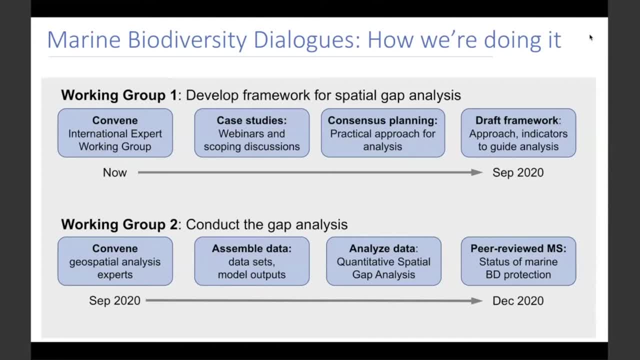 So just to come back to the first working group, which is underway right now, we've convened the group and we're starting by studying a number of specific cases of conservation planning and biodiversity monitoring that have been done and developing that as a group into a practical approach via a consensus process. 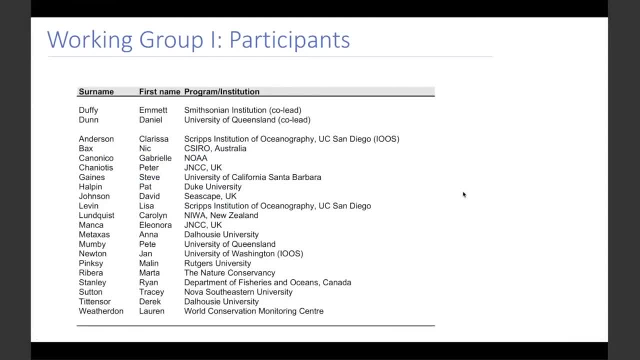 So these are the participants in the first working group that is underway. now I won't go through the group in detail, except to say that we have both scientists working in the marine realm and various different aspects of oceanography and marine ecology, as well as conservation practitioners. 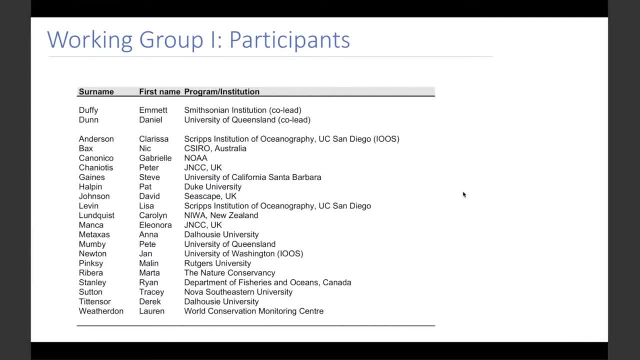 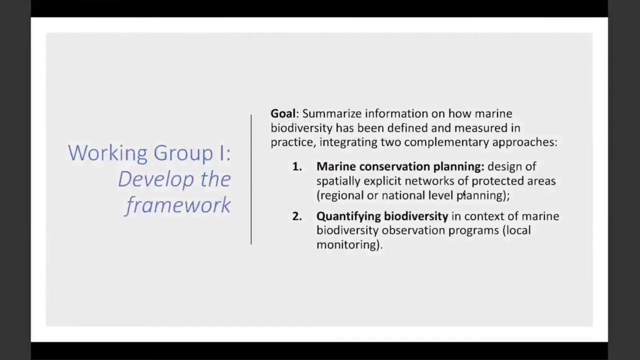 We have people from several places throughout the world with experience in different regions, NGOs, as well as academics And government scientists, And we have connections to several of the major biodiversity monitoring programs worldwide and conservation groups. So I mentioned that the first working group's charge is to develop the framework. 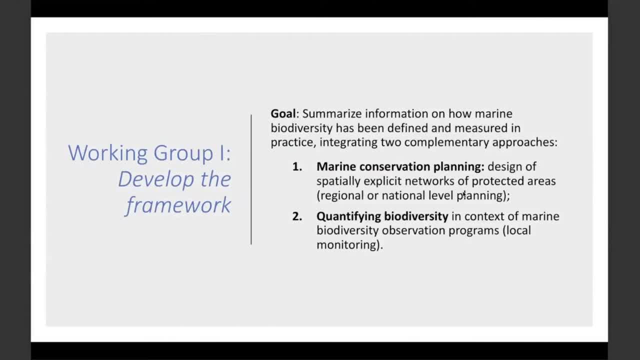 So, again, this is summarizing the information on how biodiversity has been defined and measured in practice by integrating the two complementary approaches: The marine conservation planning that we think of as something of a top-down approach that is coming from a national or regional or even global scale. 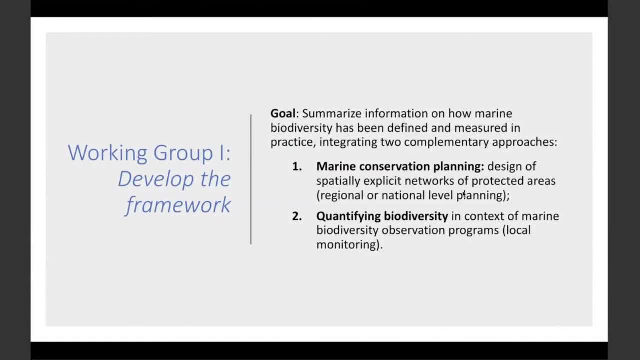 and asking how we create networks of protected areas, And then, secondly, coming from the bottom up, in the form of programs that have been focused on monitoring and describing biodiversity around the world. So we're looking for the sweet spot where those two meet. 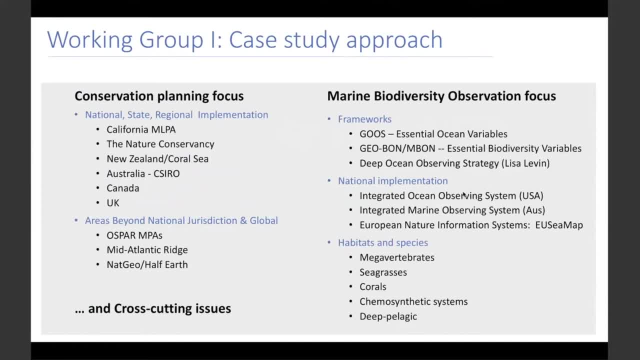 And without going into a lot of details about this case study approach, I'll just mention that we have divided our different case studies roughly equally into talks by members of the working group that have done conservation planning on national, state, regional scales. California ML. 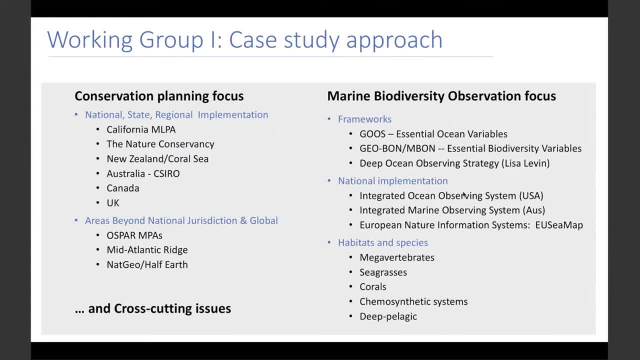 marine life protected area, for example, Nature Conservancy's work comprehensive national levels in Australia and New Zealand, as well as areas beyond national jurisdiction for the larger migratory species especially. And then, on the other side, we are hearing from experts on frameworks for marine biodiversity observation. 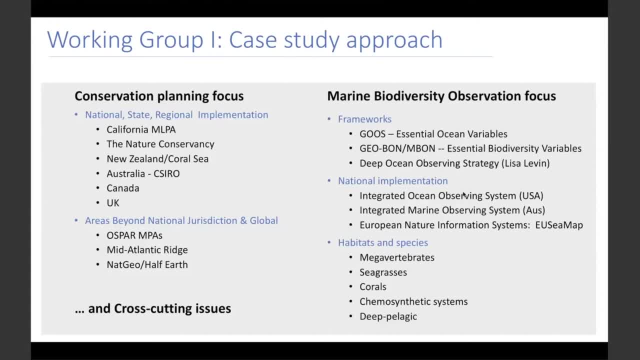 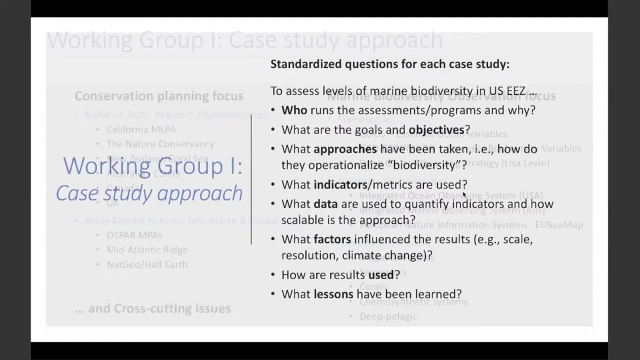 at global and regional scales, national scales, national implementation of monitoring programs and also on particular kinds of habitats and species that figure largely in these programs. So each of these, we have asked each of the speakers in this series to address a standardized set of questions. 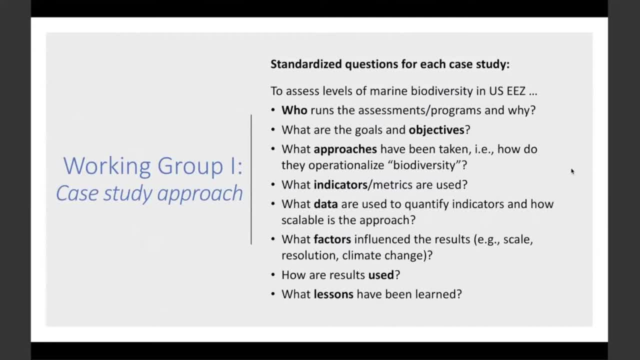 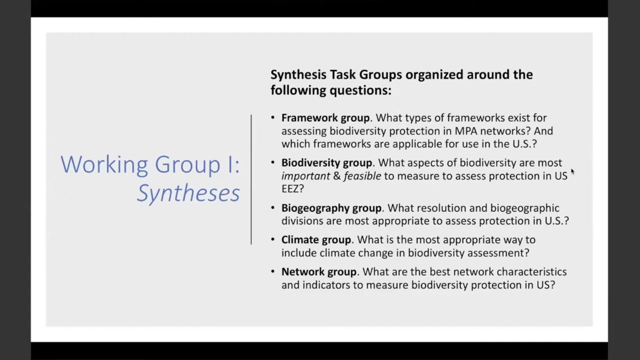 that we hope will allow us to have some continuity across them. Who runs the assessments, What were the goals and objectives, What approaches have been used, Indicators, data and what lessons have been learned, And the end product for the first working group is to synthesize all of that information into the framework. 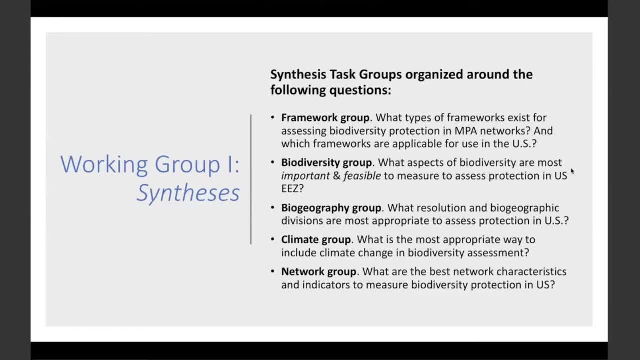 And in order to make sure that we have accounted for the different aspects of the framework that we feel are important, we have organized the group into subgroups to consider the information that we have heard and the lessons learned in terms of thinking about the kinds of frameworks that might be implemented in the United States. 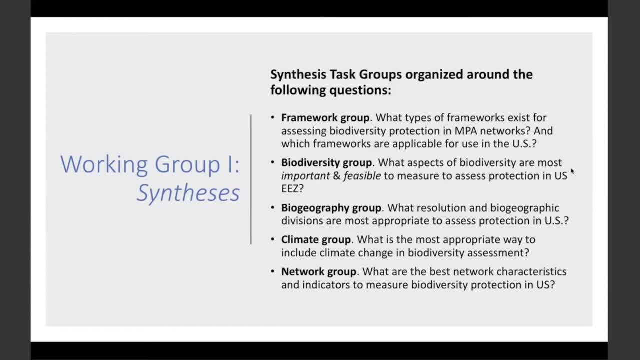 or that are most effective. What components of biodiversity are most important and feasible to measure. What spatial and biogeographic resolution is needed. How we design the process in the most appropriate way to deal with ongoing climate change. And then, finally, how we consider networking these together. 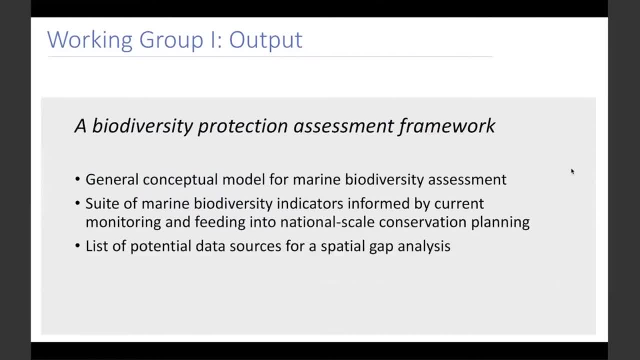 So, with all of that done, the output becomes the biodiversity protection assessment framework, And this we anticipate at this stage could include a general conceptual model framework for how marine biodiversity might best be assessed, a suite of indicators informed by what we know from current monitoring and planning. 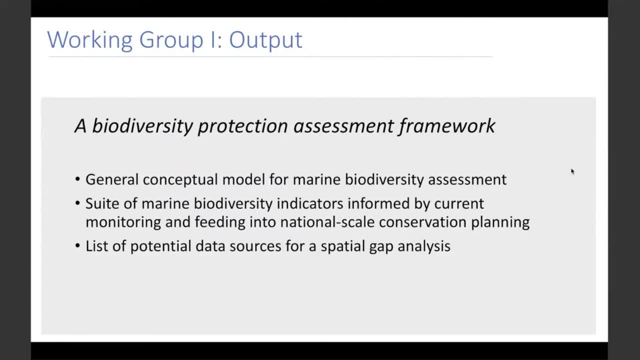 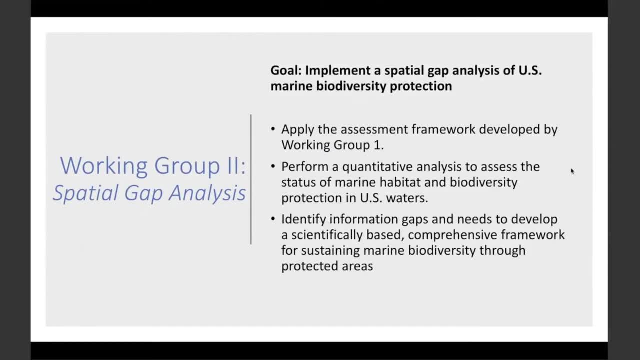 and, very importantly, a list of potential data sources that the second group will then be able to use in the gap analysis. And with that we move on to the second working group, And here I'd like to turn the podium, as it were. 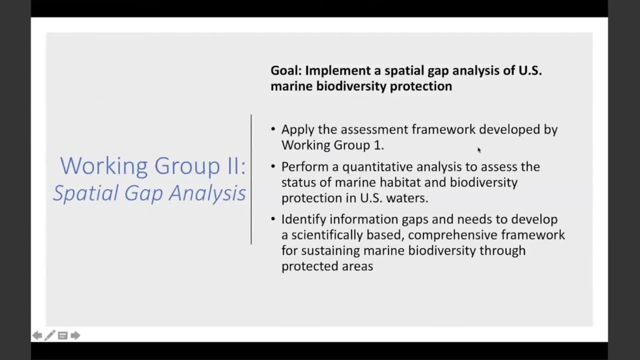 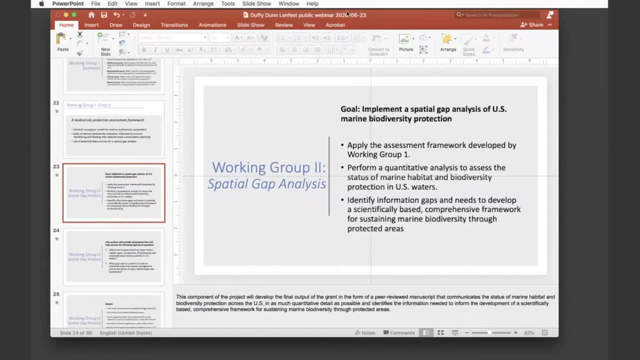 over to Daniel, who is the expert here, And I think, in order to do that I'm going to, You're good, I'll just ask you to forward the slide. Okay, good, Sorry, Let me. I was wondering if we could hear you or not. 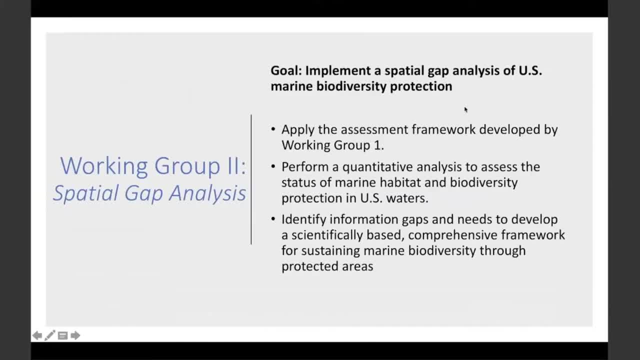 Okay, go ahead, Daniel, Yeah, Okay. So first of all, thank you everybody for joining this call. Part of the reason that you are hearing this at 7 pm is that I live in Australia. I moved over here last year from the US. 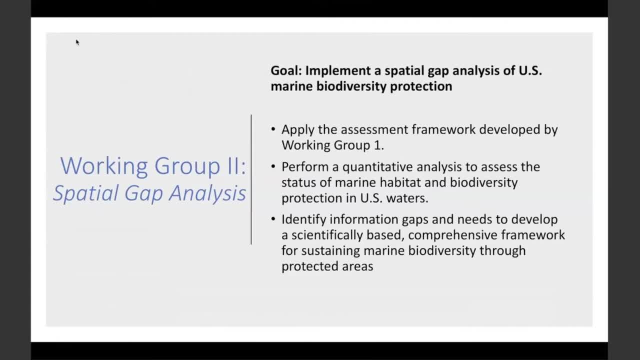 where I was working at Duke University and I now work at the University of Queensland, So I appreciate you all joining from your after hours. I'm sure there are a lot of folks in this side of the world that appreciate the ability to actually participate in this type of webinar. 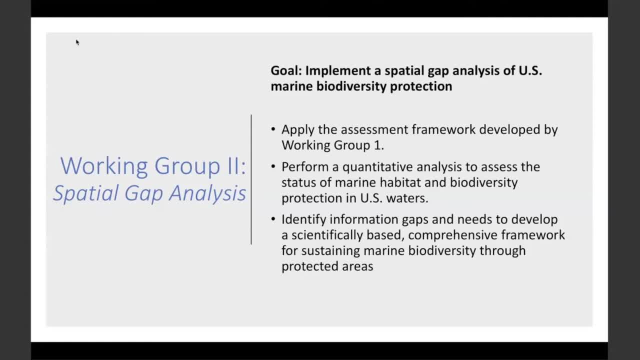 So thank you very much for joining, As Emmet said, with the working group one. these working groups are really an opportunity to bring people together with expertise on these particular matters And again, it's not myself and Emmet trying to push this forward. 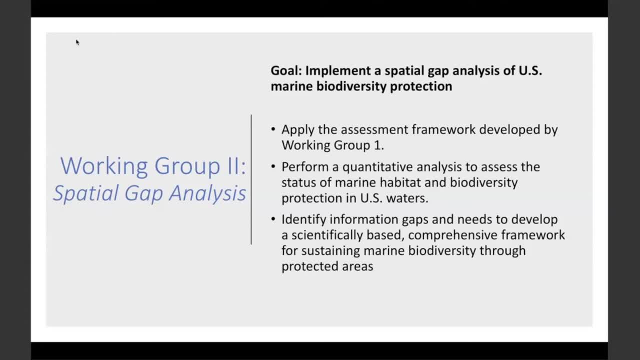 It's us trying to convince as many Brilliant Minds as we can to participate and help us with this And, in particular, working group two has not actually been completely formulated yet. There will be some people from working group one, but I suspect we will be reaching out. 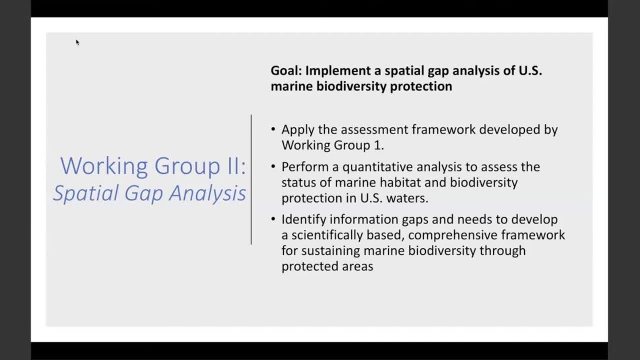 To some of the folks even on this call to actually implement, which brings me to this slide. So the goal of this is to actually implement the spatial gap analysis of US marine biodiversity protection to apply the framework that is developed by the first working group. 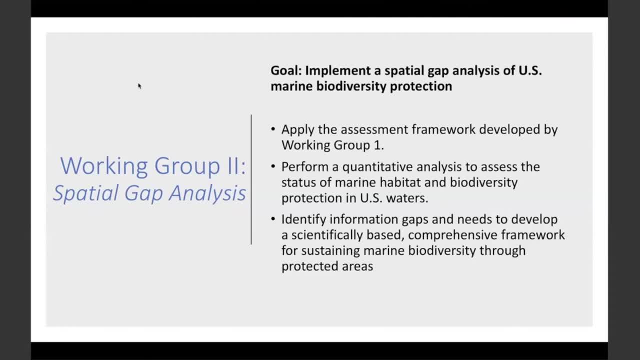 And essentially what that's meant to be is a quantitative analysis of the status of marine habitat biodiversity protection. There's been a little bit of discussion about whether this is for the inventory or whether it's a gap analysis, And the major difference between those is that a gap analysis assumes that we know what the values of the society are and what society wants. 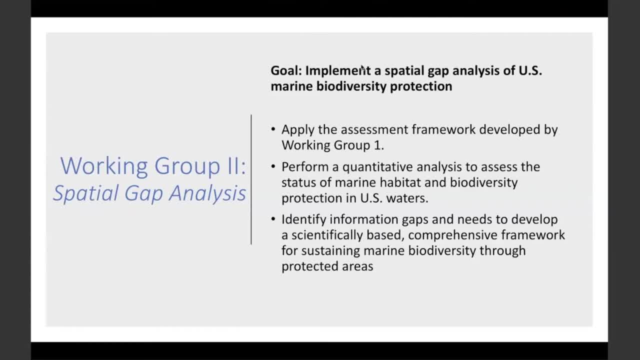 And unfortunately, we're humble enough to know that. we don't know that. And this is an iterative process And the work that's being done here, even this gap analysis, is making some assumptions about those values and is really meant to be the first step. 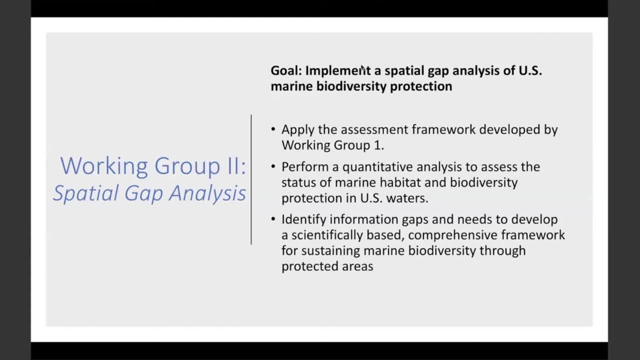 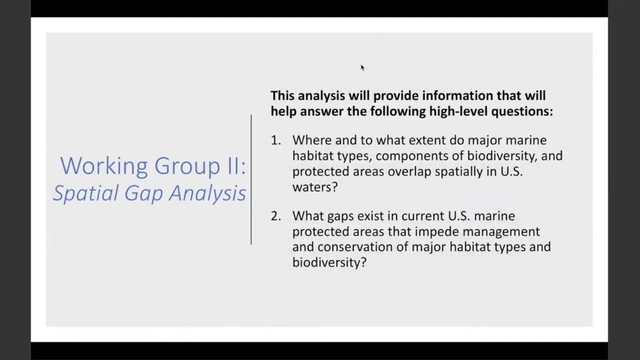 This is a first step, or a step in the process of better understanding our protected area network and where it can go from here. So with that we can go to the next slide. There are essentially two- just to put this more broadly, two main questions that we're looking at. 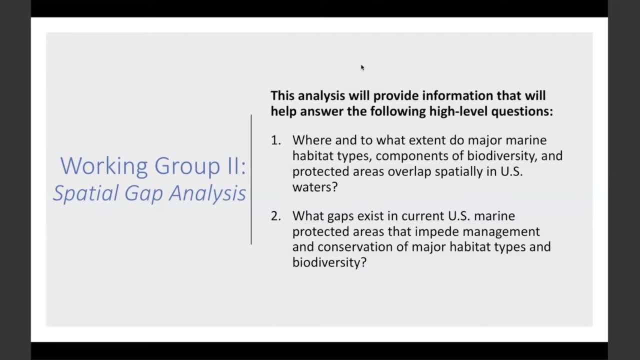 Where and to what extent do the marine habitats and components of biodiversity and protected areas overlap In US waters? And that takes away again the scope of this. We are talking about all US waters, which is pretty intimidating. 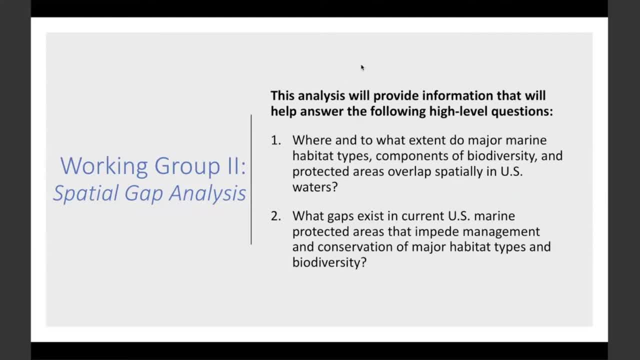 But that is the intent. And then again, what gaps exist within the current protection And those gaps? we're really thinking about it from an ecological perspective. Chris, at the beginning of this webinar, indicated that there are ecological gaps and there are management gaps. 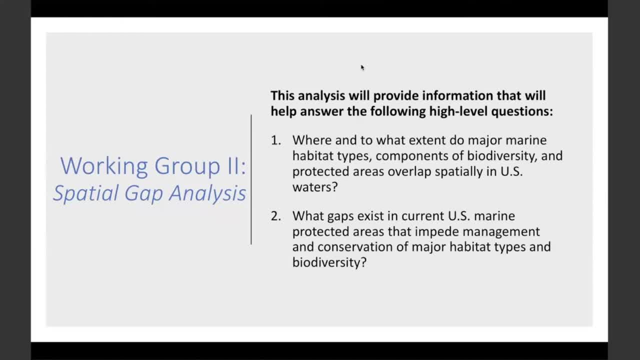 At this point we're trying to stay away from subjective or any really interpretation of the levels of protection that are offered to different habitats in terms of what the different management measures might provide, But so we're looking more at an inventory of just what's in the variance types of management measures. 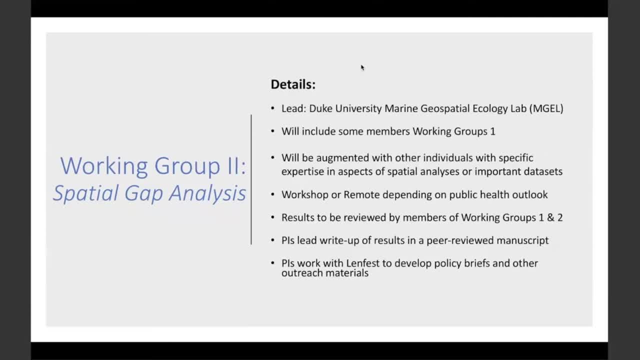 We go on to the next slide, which I believe is the last one on this. So the details on this is that the actual analysis will be led By the Duke University Marine Geospatial Ecology Lab. The working group will consist of about 10 people. 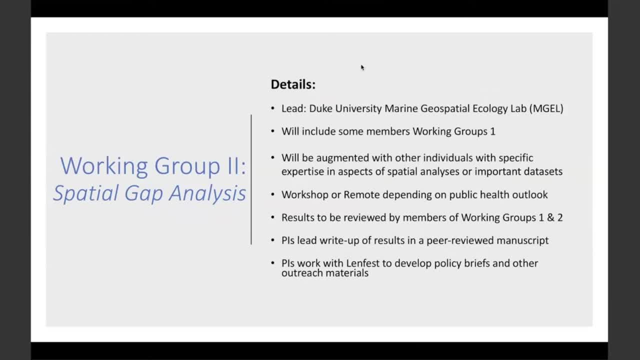 I believe we're thinking at this point in time. Some of those will be from members from working group one to provide some continuity, But that will be augmented by folks, like I said, outside with expertise on spatial analyses and maybe specific data sets that we'll need to bring into the analysis and just general expertise on the subject. 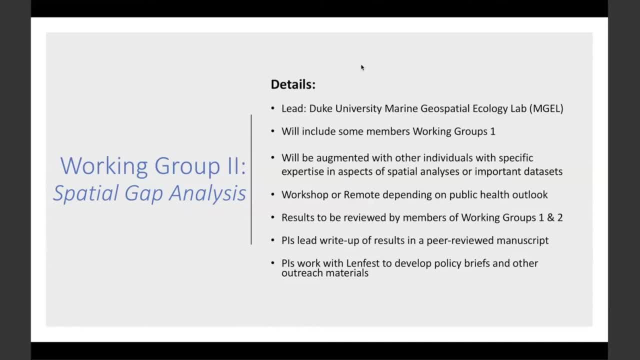 Originally. I don't think we've mentioned this, but this entire effort working group was meant to be two week long workshops. Obviously, with the current public health outlook that is not possible at the moment And we'll see whether it's possible for us to do this analysis over a week long workshop or whether that will be done remotely. 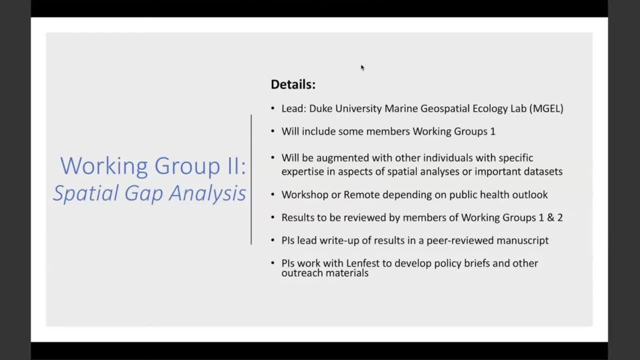 I think we're all getting pretty used to this remote method of communicating. There will be an opportunity for review of the output, both by working groups, by both working groups, as well as an opportunity for feedback input from a broader community as well. 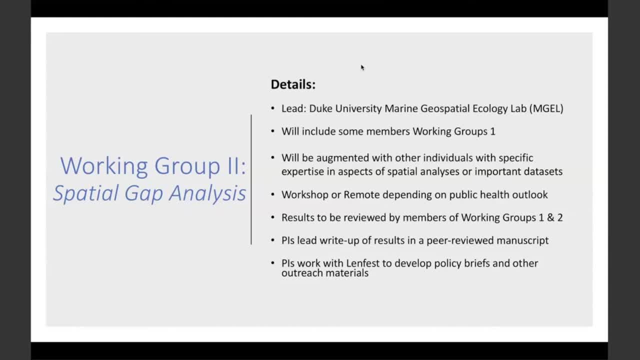 at which point we will continue writing out the results in a manuscript. And one really exciting element of this for us, like we said at the beginning, is we do want this to make a difference. We are really excited that this project was essentially 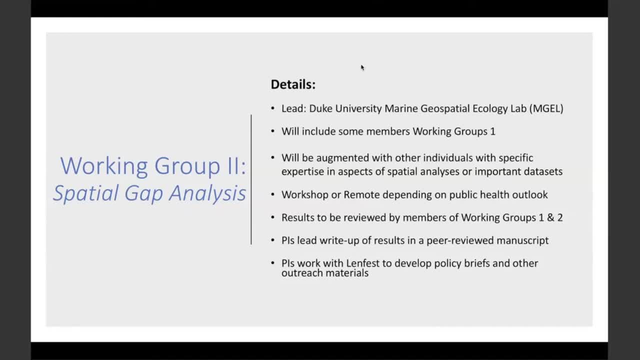 the ball got started rolling through requests from Chris at the National Marine Sanctuary Foundation to provide input on what levels of protection exists for biodiversity, And we really want to be able to feedback to managers. We've already had a call with managers at various agencies in the US. 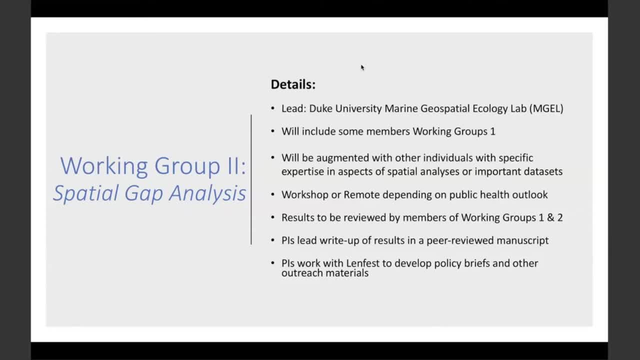 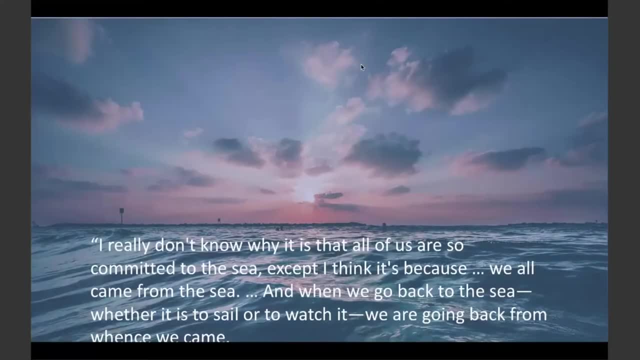 and we're very excited about working with LEMFEST to develop policy briefs and other outreach materials to get this information out as far as possible. With that, I will hand back to Emmet for the last slide. Thanks, Daniel, And it looks like I somehow got this cut off from the bottom. 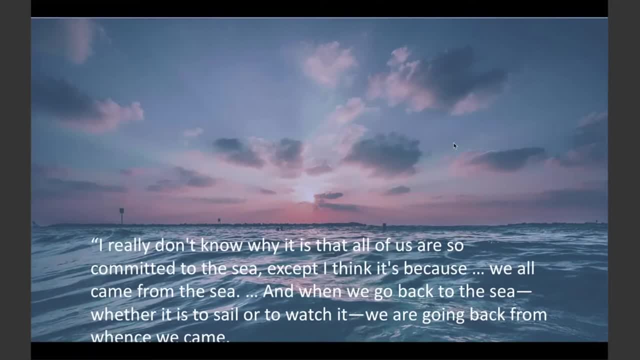 but I just wanted to end with a quote from former President Kennedy, who said that I really don't know why it is that all of us are so committed to the sea, except I think it's because we all came from the sea. And when we go back to the sea, 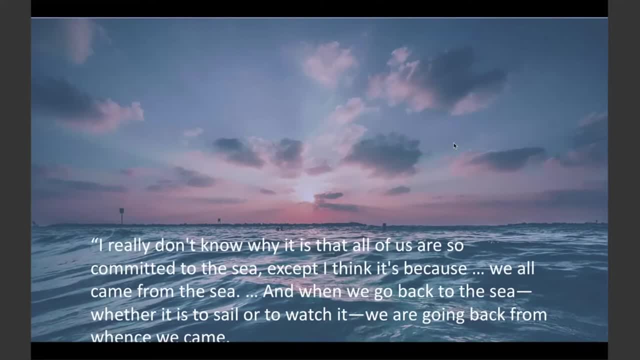 whether it's to sail or to watch it or perhaps even to fish. we are going back from whence we came, which I think is a really is a especially poetic way of saying that we really do depend on the ocean. This is now really finely documented by scientific evidence from various fields. 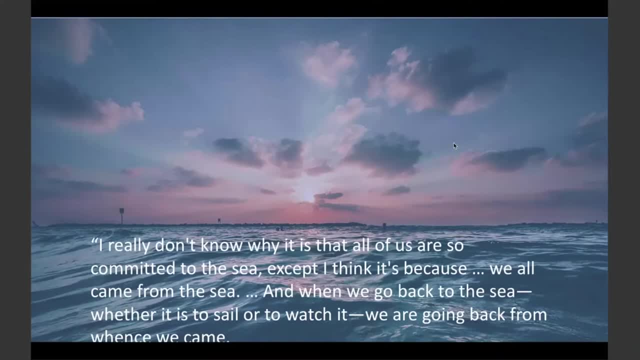 And that's part of why we're doing this- is because we understand that we depend on the ocean and the organisms are the engine of ocean ecosystems, And so that's where we're coming from, And so thanks all for listening And I think we have time for some questions. 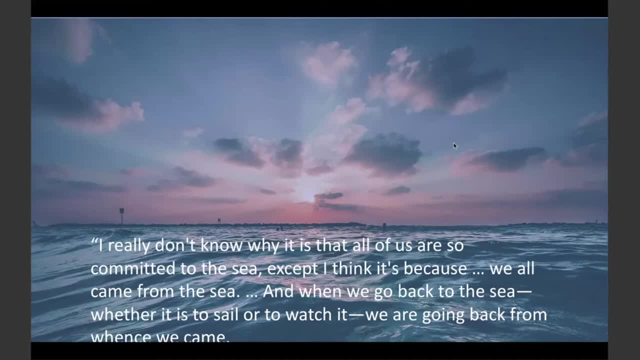 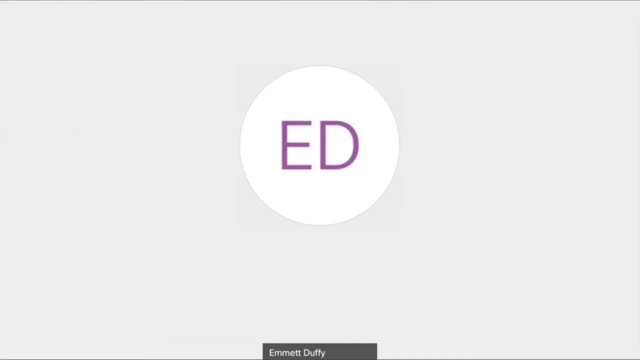 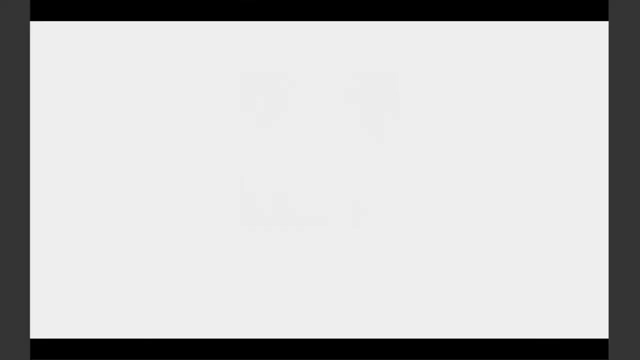 I'll turn it back over to Emily here. There we are All right. Thank you so much. So, yes, So I'm going to quickly, quickly share my screen, for So folks see the ending, the ending slide which reminds us to: 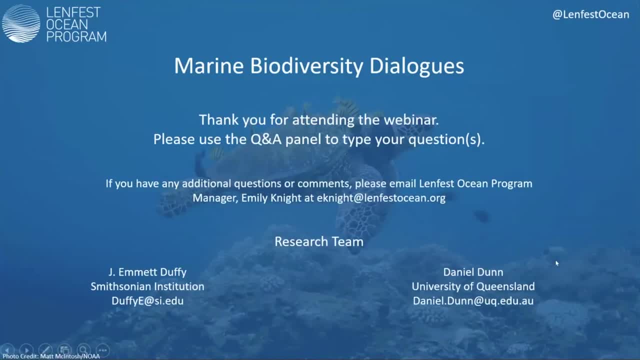 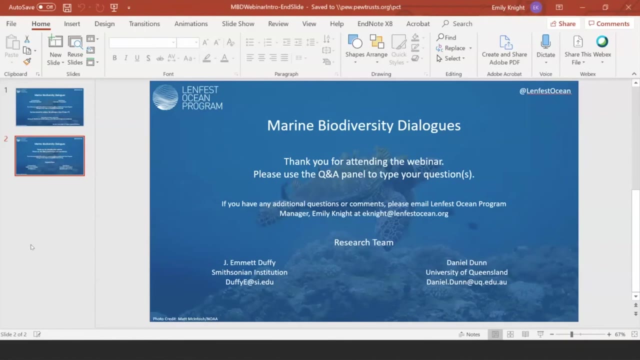 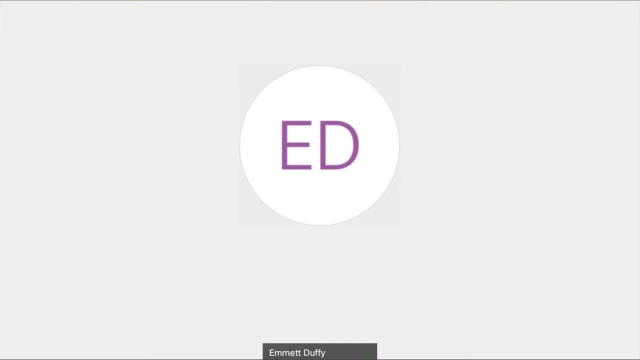 if you want to ask questions, please type them into the Q and a panel And I will read them from there, And we do. we have about 20 minutes for questions. Okay, Let me make sure I'm seeing everything, Okay. 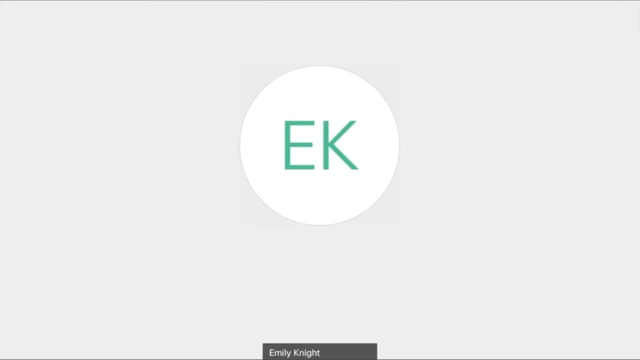 I'm making sure I'm seeing. I'm actually seeing the Q and a panel. Okay, So the first question that we have is And and not And. I'm not sure, at Emmett and Daniel, that you'll necessary that you will have an answer to this. 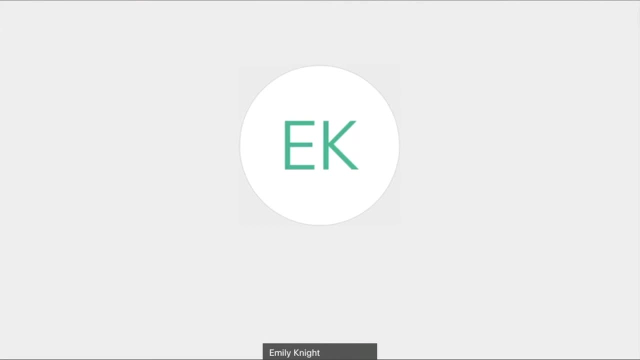 but I do want to read it out loud. Um, and to be clear, this project is about assessing marine biodiversity in U S waters, But are there any talks about collaborating with the Canadian government to make the Bay of Fundy a conservation area? 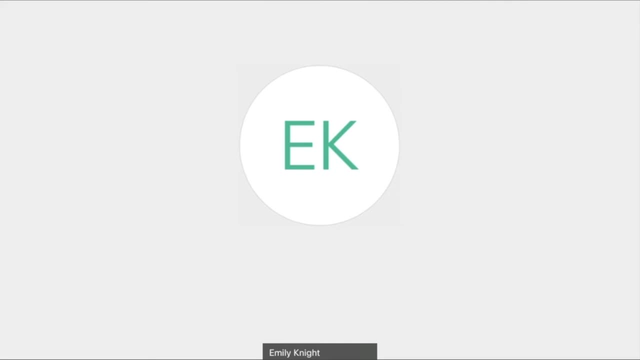 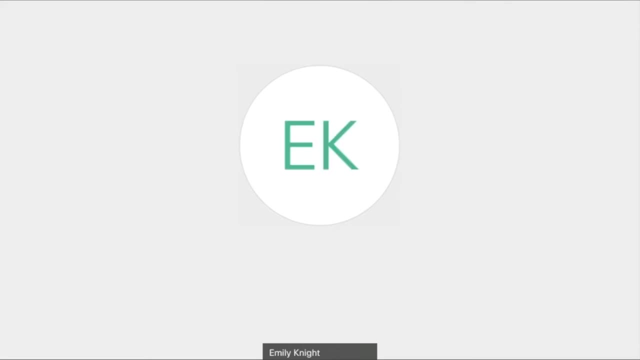 Oh, I thought there was a question here. Did we do get that? Yeah, this question is going to go to Daniel. Daniel, we can hear you very well. You can't hear me very well. Can you hear me better now? 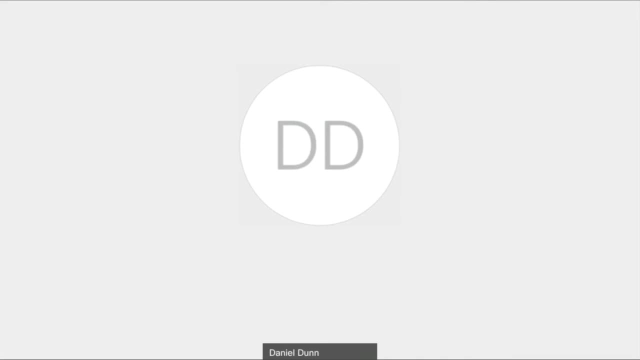 Yep, That's good, Now we can hear you. Yeah, Sorry, That's definitely beyond the geographic scope. I mean, obviously the areas are related and connected. speak to that. There might be people on the call who can. I've seen at least one person. 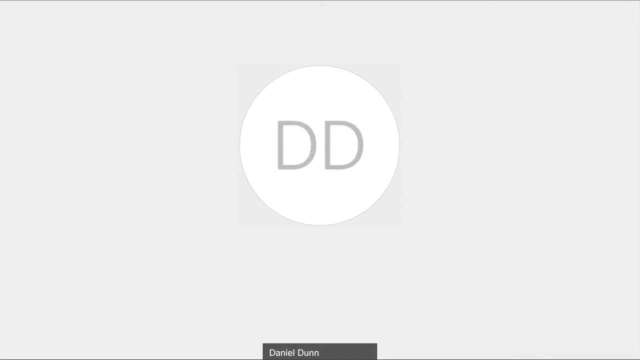 from that region. Fred Roeske's up there who might be able to give you some information on that, but I don't think we can answer that question. Yeah, I'll only add that we definitely have experts, as we mentioned, from various countries. 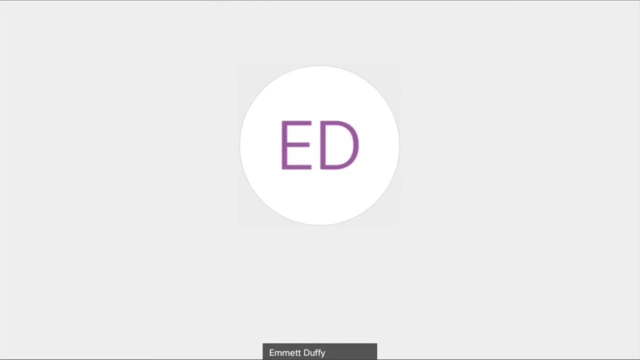 including Canada on the working group, so we're hoping to at least benefit from their experience. Yeah, that's great. I just saw a question from Sylvia in the chat. Sorry, I was trying to put it in the Q&A, but it's having difficulty. 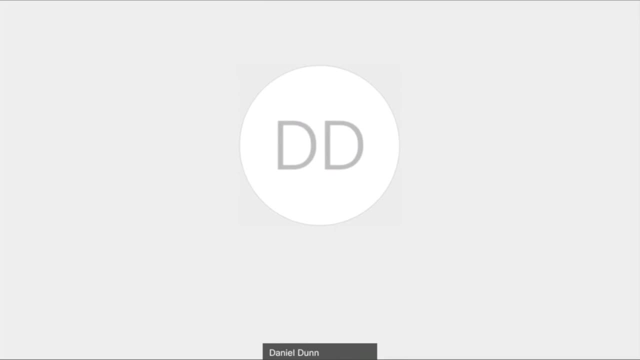 Yeah, sorry, So other people may be having difficulty with the Q&A If you do just throw it in the chat. Oh yeah, So the second question in the Q&A is: has eDNA technology started to improve understanding of ecological connectivity and distribution of biodiversity in the ocean? 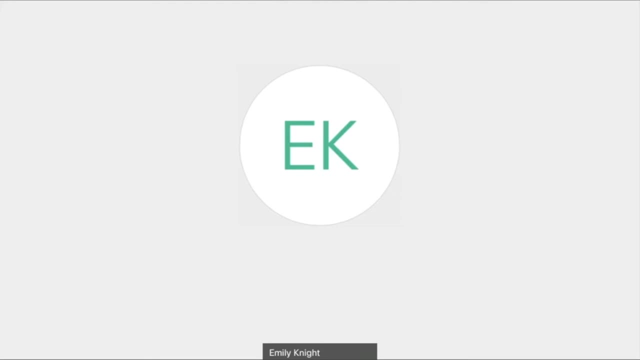 What role do you expect that technology will play in better informing global, regional and local biodiversity conservation plans? Wow, that is definitely one of the holy grail questions, so to speak, as we go forward in biodiversity research. I would say, in answer to the first question, eDNA is a very important 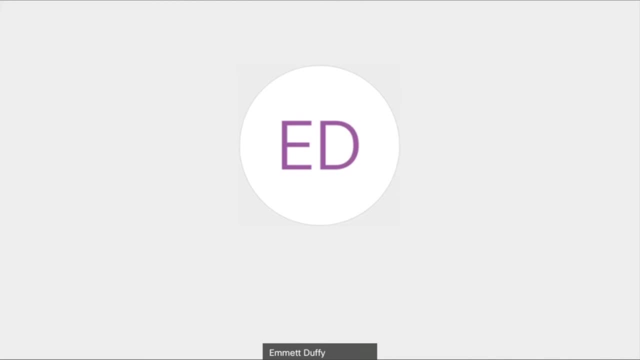 resource. It is certainly proving useful in looking at connectivity, particularly in cases where the way that DNA works for a particular organism is well known and the habitats are sampled properly. So there's a lot of promise there. There are many wrinkles to work out before. 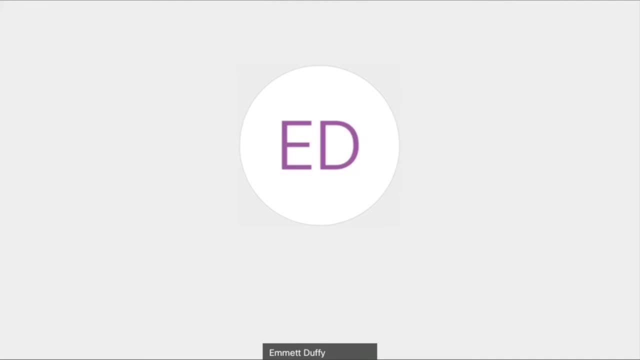 it's used very broadly, or I should say for particular questions. But I think this was an answer to the second question: eDNA, or metabarcoding, more generally, that is, or metagenomics, that is, looking at the genotypes of samples from the environment. 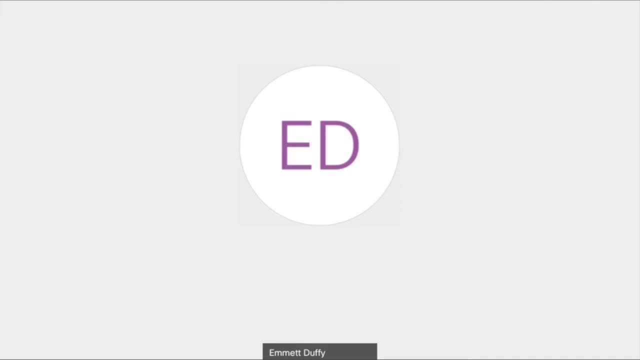 rather than from individual organisms is proving that biodiversity is much larger than we might think it is. So I think it's a very important question. I think it's a very important one to consider, And I think it's a very important question and I think it's one that we really need. 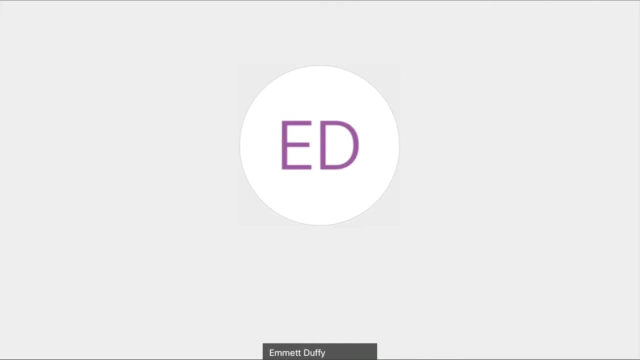 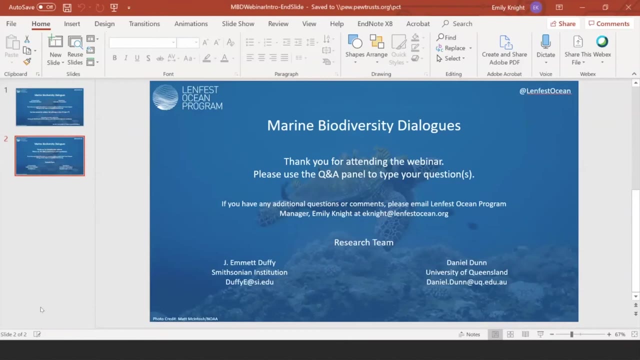 to think about, And it's a very important one to consider, I think, in terms of what we might expect from the other, from the types of samples that have traditionally been collected, And so there's tremendous interest and, I think, promise in eDNA being a key biodiversity measurement. 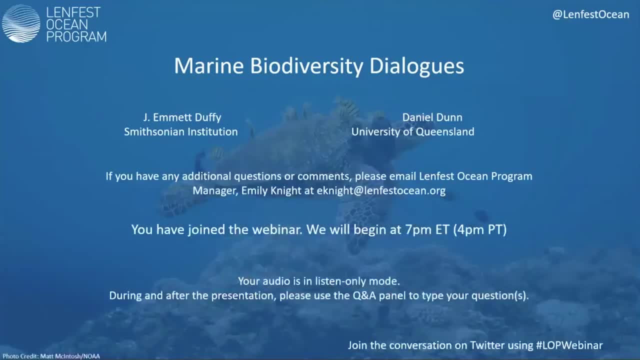 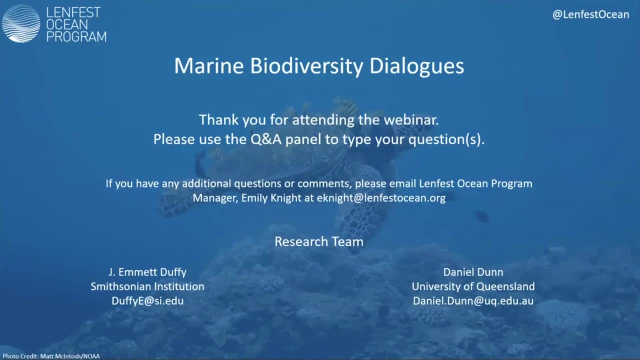 variable as we go forward. There's a lot of work left to do on what questions it can and cannot answer. well, Thank you, Thank you, John. Thanks, Thank you, Great thank you. And another question from the Q&A: what is the plan for using open access? 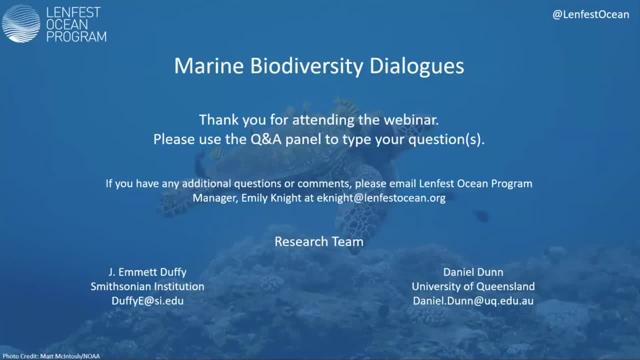 data for the spatial gap analysis and ensuring all data are openly accessible and, if possible, standardized. Yeah, I can jump in on this one. Thank you for the question, Abby. You would know the scope of the available data as well as anybody. Yeah, absolutely. First of all, the geographic. 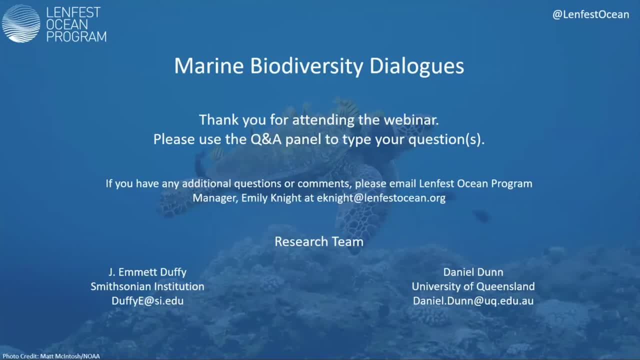 regions that we're talking about. the scope is huge, And so we really are going to be looking at regional and, in some cases, global data sets and then try to determine what's available on sort of smaller regional data sets. But we're probably going to be relying on those larger regional data sets which are 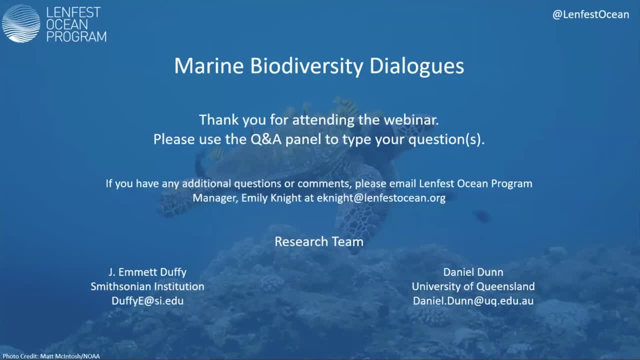 generally open access And I don't think we'll be using any proprietary data for the analyses that we're talking about, And this will actually- we'll come back to this because there's a question about the temporal nature of the analysis or when we expect to be finished. 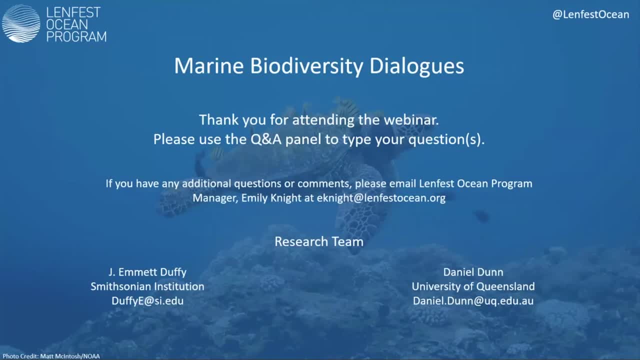 And that also feeds into this. This project is meant to be completed this year, So we're hoping to have the analysis done by the end of the year And again, to do that, we're really going to be relying on existing data sets and open access data sets. 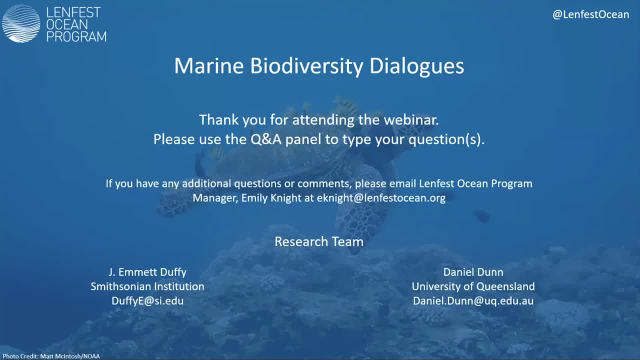 Cool, Thank you guys, And I'm going to- I'm flipping over to the chat now to make sure we capture everything- And we have a question: What is the best way to follow the progress of this work- And I can jump in at first on that and say, to follow the progress of this work please? 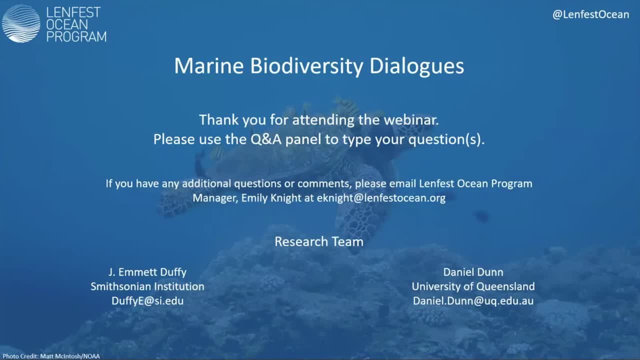 do let me know that you're interested. Honestly, we are at the point where we're sharing initial information about the work. The work is getting going right now And we intend to organize other outreach events and meetings based on what we hear from you, And I'm going to go. 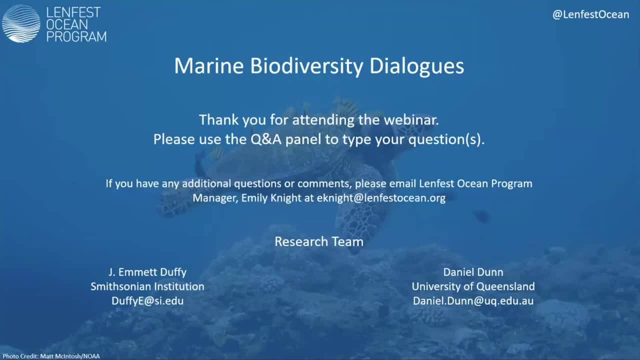 ahead and say if you have questions, please feel free to email me. We're glad to hear from people. So we kind of plan that as we go, based on what will be most useful and interesting. So feel free to reach out to me on following the progress And I will also let Emmett or 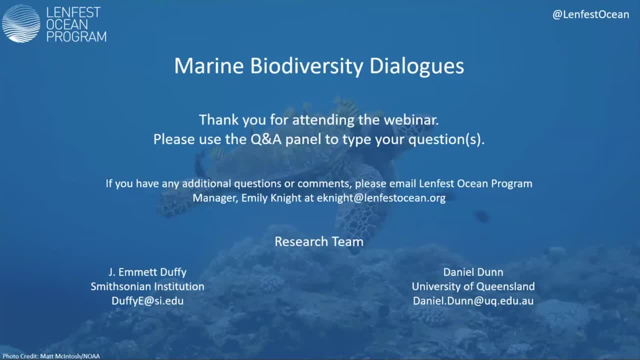 Daniel say anything more about that. I think you've captured it, Emily. We certainly are planning to work with LenFest on the work, So we're hoping to have that. Thank you, uh. outreach in in various formats. um, we, we want people to to know about this and to give us. 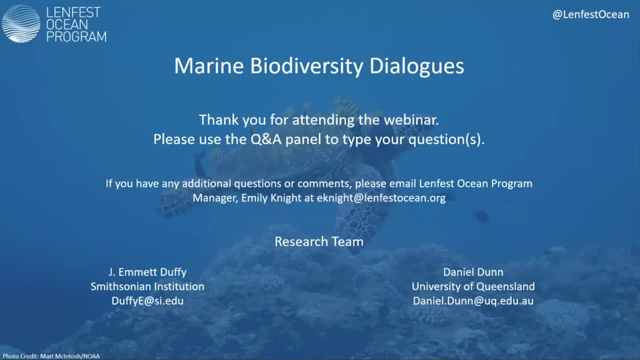 feedback. great thanks. and and then we have a another question in the chat. uh, how expansively will you define protection as in specific threats beyond just fishing, such as shipping and other industrial uses, and to what extent will you look at protected areas and estuaries which? 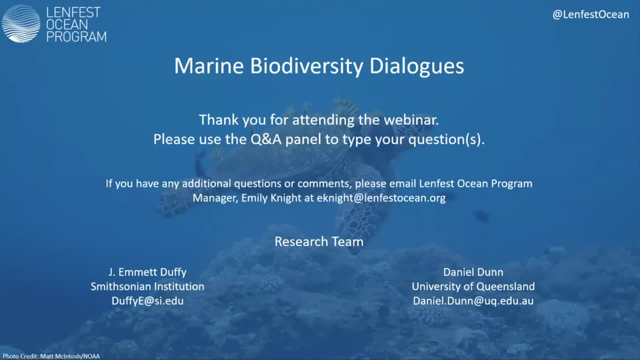 are vulnerable to indirect threats. i can, i can jump in here, but i uh and um. knowing emmett's expertise will help um you decide as to whether or not we will be focused on estuaries. given that he is a seagrass ecologist, i suspect it would be impossible for us to remove those areas. 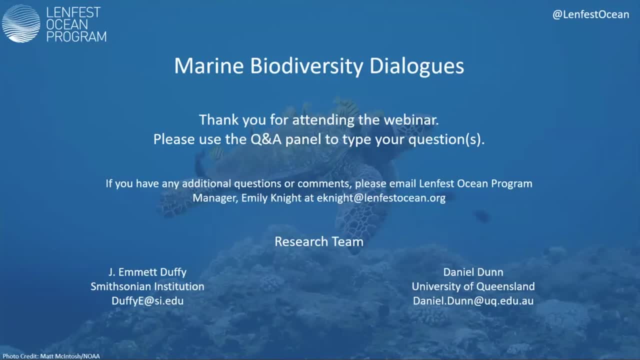 from this analysis, um, so definitely on the on the estuary side and with respect to how we define um protections, i mean, i think we're what we're looking at is is areas that have been designated by um the government right? so we're not, we're not determining based on um threat status, uh. 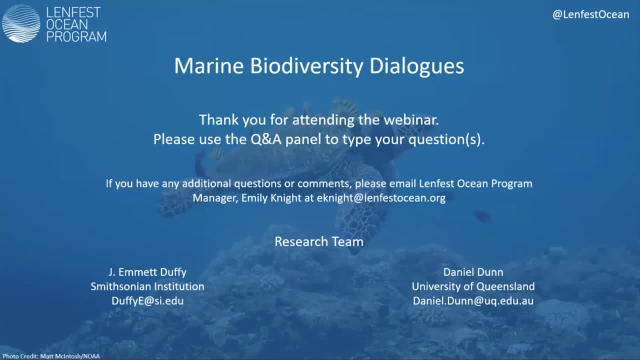 areas that should be protected. we're looking at things that currently have some level of designation by um, the, the government, um- and then trying to take an inventory of what's in those areas, so we'll get you back to you there within just a matter of minutes. 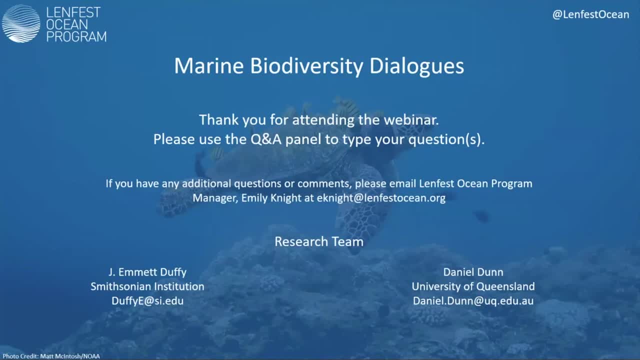 yes, and, as daniel mentioned in in a previous comment, we, given the time frame especially, we're going to really have to rely a lot on publicly available and easily accessible savings and, um, some of that is from estuaries. uh, you know, estuaries are really where humans are concentrated. 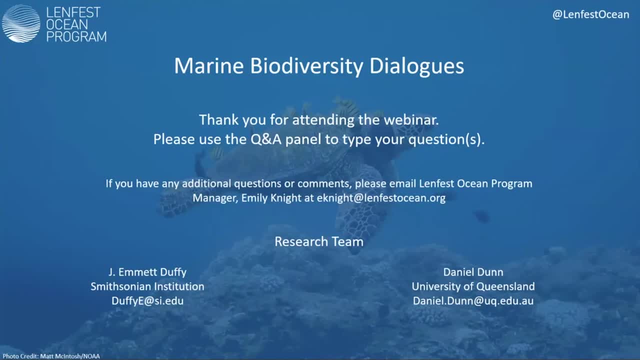 and so to the extent that that we have uh protected areas in in estuaries and certainly be key parts of our work, Cool, thank you. We have another question here, going back over to the Q&A: Are you hoping to use this research? 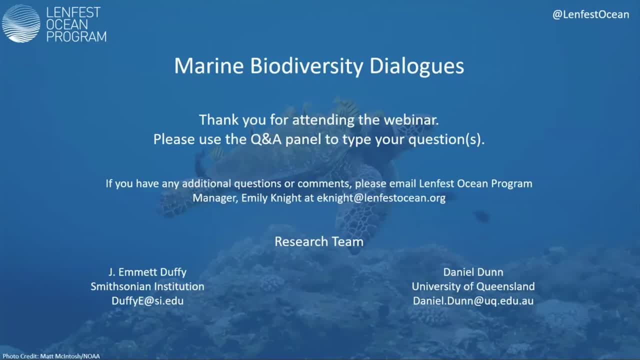 to contribute to the 30 by 30 mission. Well, I would reiterate here that our goal is to provide the data and the information and framework and interpretation that will allow planning of new and existing protected areas or management of that network. So in that sense, 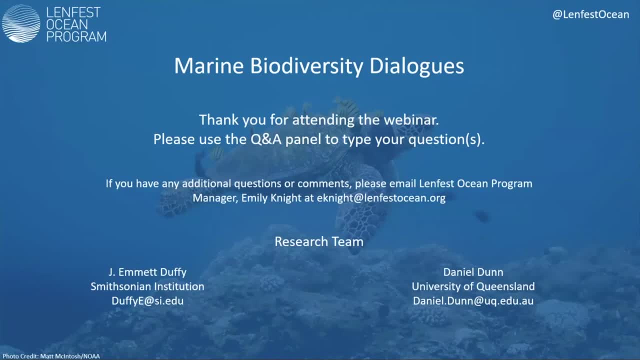 we are officially agnostic to contributing to that, but, needless to say, the whole point of doing this kind of work is for better and more effective and sustainable protection, And so, in my opinion, that sense, I think you know, on a personal level, I would certainly like to see this. 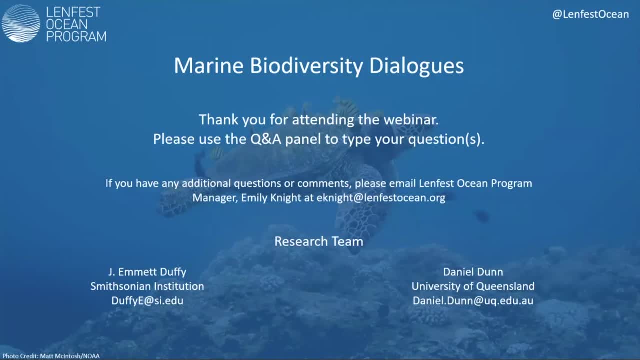 contribute that way. Yeah, and I think it was probably informative to hear Chris's introduction and talking about how this information is relevant for expanding the current system of areas under some level of protection in the US. so I think that concept was sort of contained within her original. 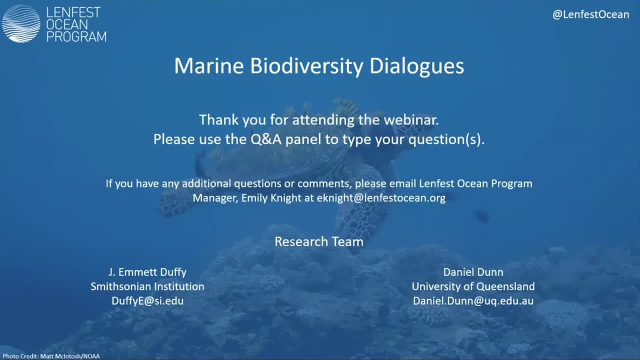 question. so that would necessarily feed up into any efforts at achieving 30 by 30. Cool, Thank you. And we have another question. This is an impressive amount of analysis. In what form will you present the results and how will the results be shared? 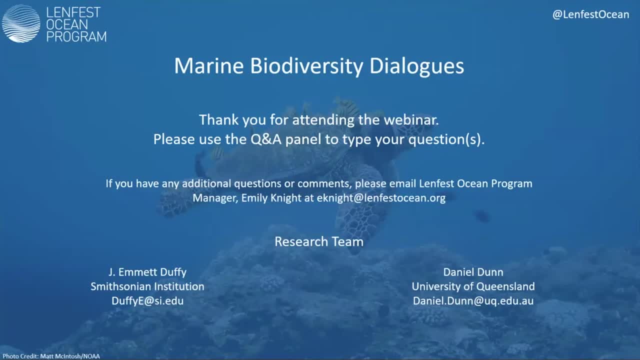 Do you have a goal date for presenting results? Well, the project is in…. It's intended to be completed by the end of this calendar year, which is seeming closer all the time, and so that answers the question about the goal date. I mean, it could very well be some months after that before we have the, you know the. 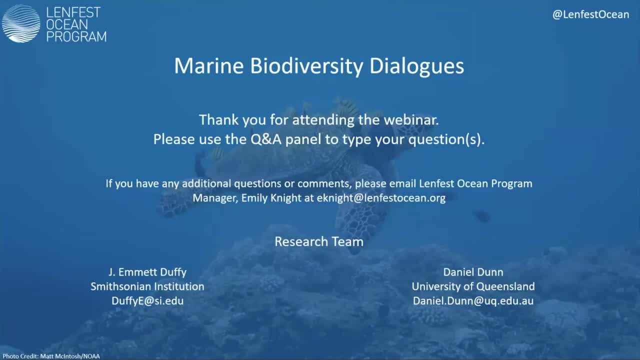 final products completed. but in general, I would say, you know, we plan to publish the results in the peer-reviewed literature, preferably open access and…but also you know… So, again, given that the data are likely to be largely open access, we expect that. 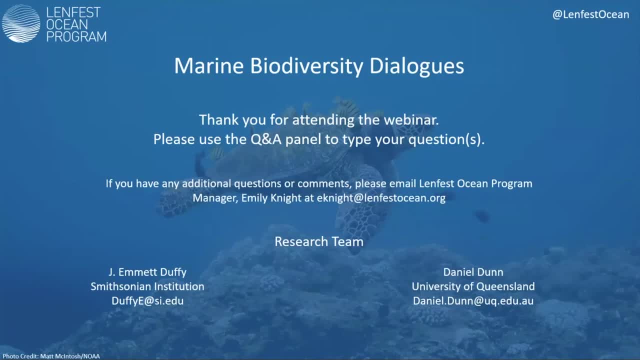 the products from those…the synthetic, synthesized products of those data, I would think would also be open access, Daniel, anything to add to that? No, I agree with all of that. Cool. So we have another question here. The concept of dynamic ocean management addresses how to monitor and manage biodiversity in 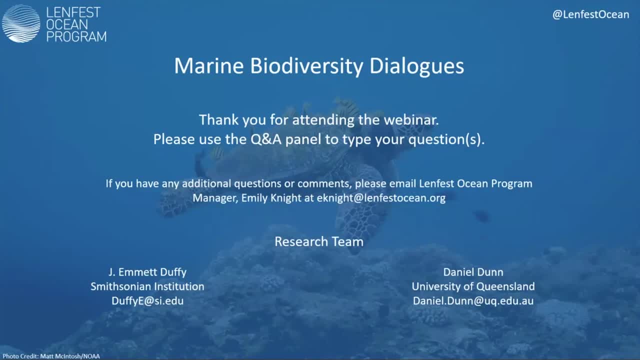 environments where oceanography and species distribution are highly variable in space and time? Will the project consider existing or prospective DOM efforts or dynamic ocean management efforts? That one's definitely got you written on it. Yeah, Okay, Daniel, Yeah Yeah. This is one that's close to my heart and it's a great question. 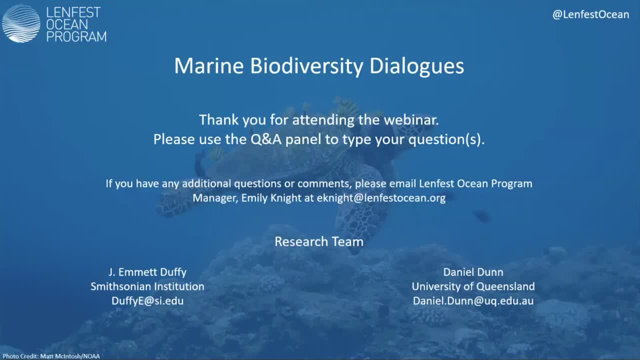 Most of the…all of the efforts towards dynamic ocean management within the US have been sectoral efforts. right There are fisheries. There is at least one example of trying to work with shipping lanes in a dynamic manner. We are not sort of nationally designated cross-sectoral measures. 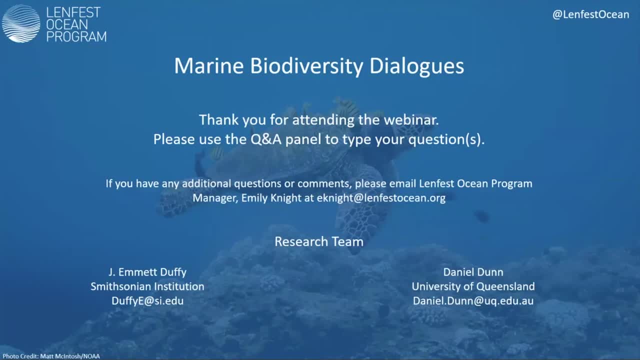 So I think we are very interested in this question. I don't know that any of those designations would fall within the scope of the designations we're currently thinking about looking at, but it's definitely one to keep on the list and to try to think about how we're going to address not just dynamic ocean management. 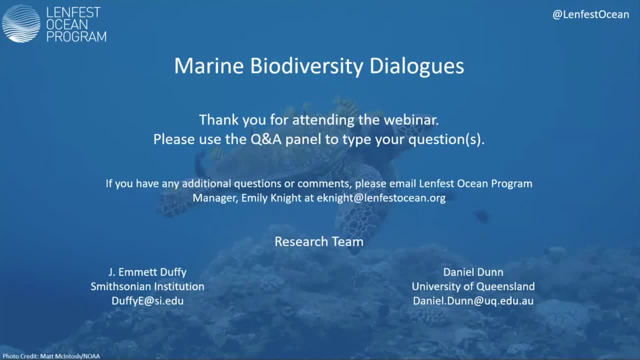 but those sectoral… the protection offered by sectoral management measures? Awesome, Thank you. We have another question: How do you envisage to account for species for which there is not enough spatial data or only point data? That's another great question. 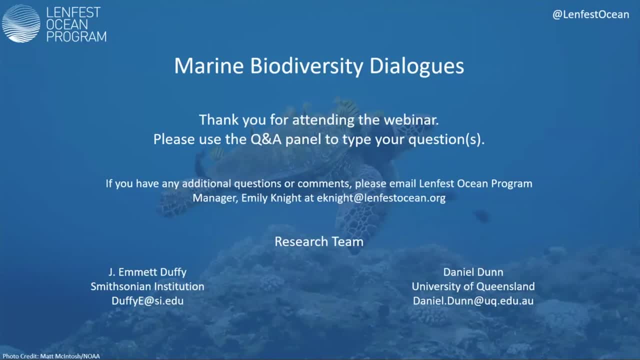 Yeah, it's…in terms of running prioritization efforts, those places where you only have a single point is impossible to incorporate into any type of prioritization, because you just end up selecting those particular areas every single time, So you can't…in the same way, it's extraordinarily difficult to think about a gap analysis where 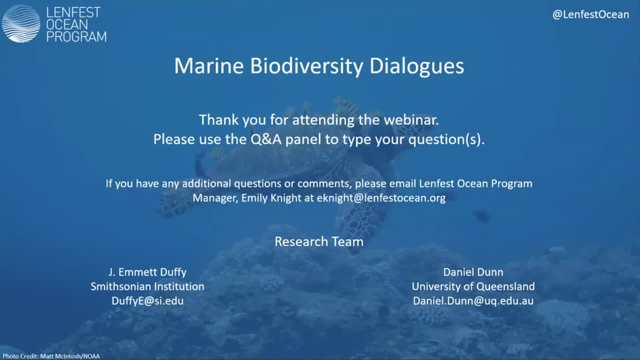 you're trying to make sure you've got each of those species where there's only a single point. This happens a lot of time in conservation planning- right where you have a rare species that the last sighting was in 1956, and what do you do with that single point? 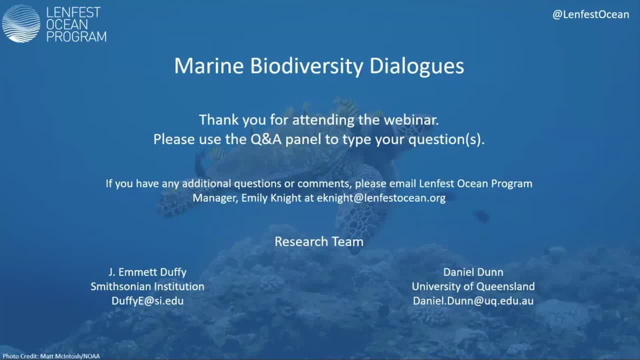 So I think, right now, the general idea is that there are going to be charismatic species which are generally a focus of conservation efforts, which we'll be able to include because we have enough data or models to include them, Right, Okay. And then, where we don't, the…generally, the idea is to move to proxies of biodiversity. 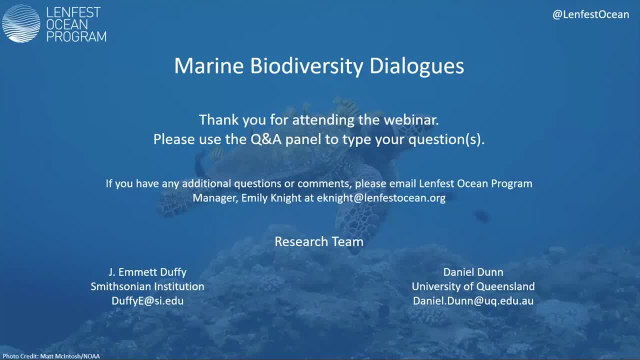 in general. Great Thank you. And another question: are you going to account for the historical distribution of species or the recent distribution slash recent records in your gap analysis? Okay, This is probably most appropriate for Daniel too, but I'll give him a break. 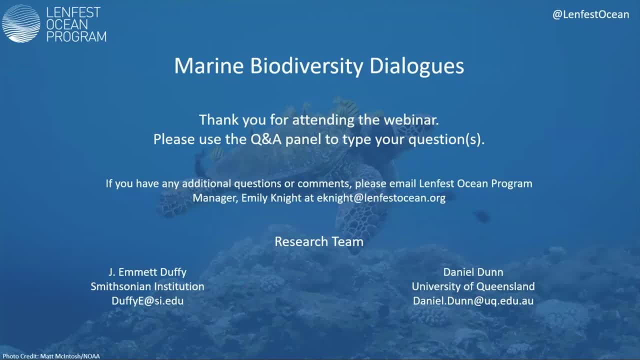 So you know, I think that the answer is actually related to Daniel's answer to the last question, which is: you know that oftentimes the historical data will be even spottier than current data. And so, you know, without a really strong reason…and sometimes there are strong reasons- 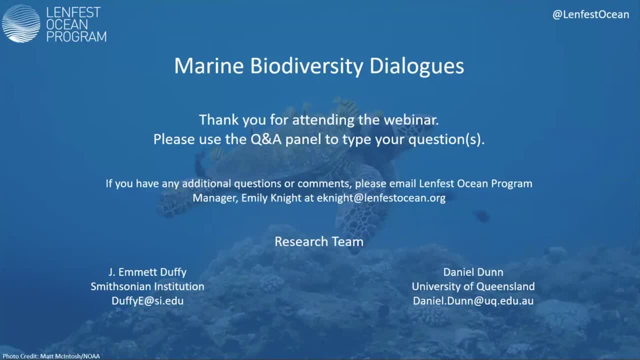 for, you know, looking into the historical data. Okay, So you know, if you look into the historic occurrence of species, I think we'll most likely be restricted to relatively current data. And you know, even within that constraint, the data will have been collected at various 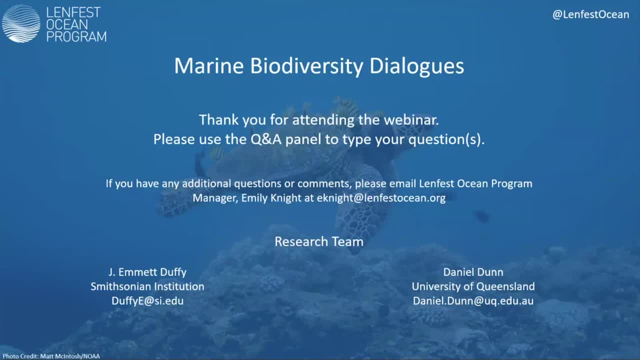 different times, you know, over the course of years. So most likely the data that we use will primarily be relatively recent. I don't know, Daniel, is that fair? Yeah, I think that's fair. I mean, I think actually what we've been thinking of more is the sort of rapid recent changes. 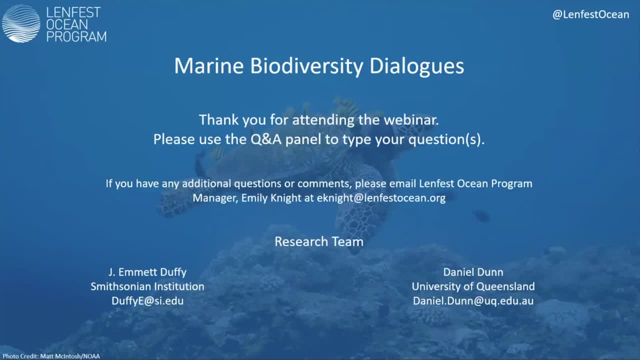 that are going on, such that the data that you have for the last decade might not actually be useful for the next decade, And in that case we have spent a fair amount of time and thought trying to make sure we have experts within our group that are focused on things like climate velocity and climate. 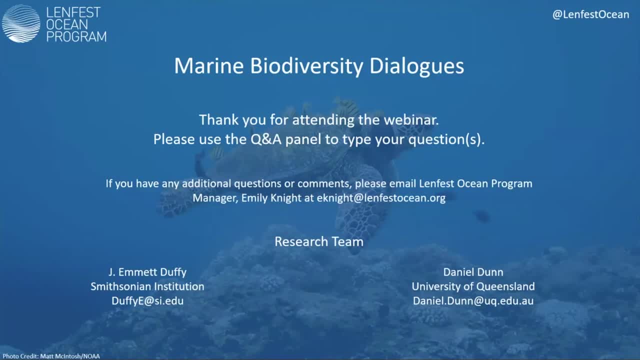 trajectory and how we can incorporate those to make sure that we are not just assessing gaps currently, but gaps in the near future as species move. I guess I can add one more thing to that. I do think it's a really good question in terms of thinking about restoration efforts. 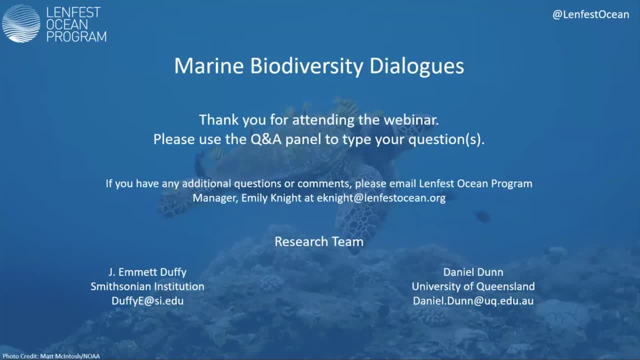 and trying to restore species ranges to places where they used to be but where we're currently not seeing them. Okay, I think that restoration has not necessarily been an objective of this gap analysis, but I think it is a really good point to raise as to how we envisage this, complementing or 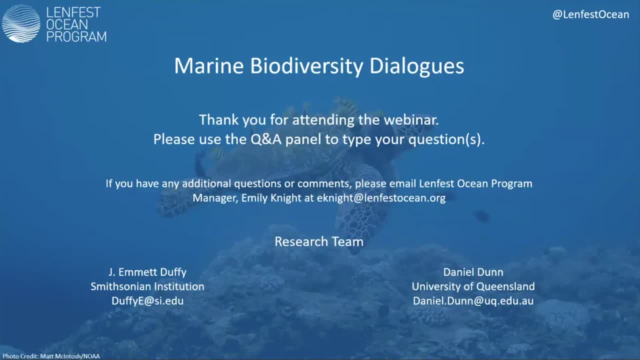 feeding into any thoughts about areas to be restored. Great, Thank you so much, And we've got a couple more questions here. I'm curious if there will be a complement. I'm curious if there will be a complementary effort to map the footprint of ocean uses. 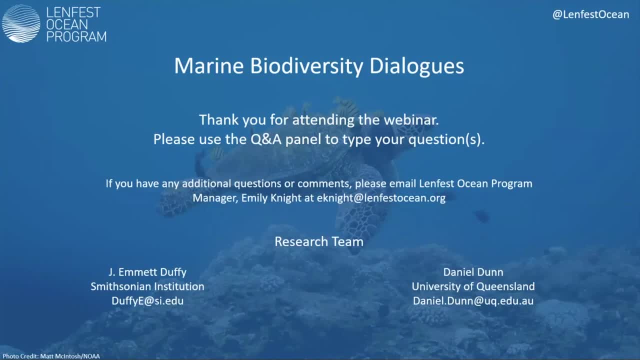 that could help assess potential threats to biodiversity. And obviously you know we at LENFEST are not funding a complementary effort. but I wonder, Emmett and Daniel, if you want to speak to how impacts from ocean uses will, you know, interact with how you assess biodiversity in this project? 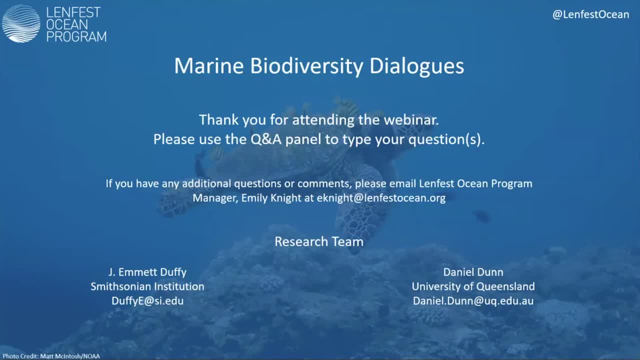 I can jump in and Emmett can correct me. he's the federal employee, I'm not, so there's probably differences in how we would are allowed to answer these questions or a federally affiliated employee. So the first answer is, as Emily indicated, is that it's not part of this project. 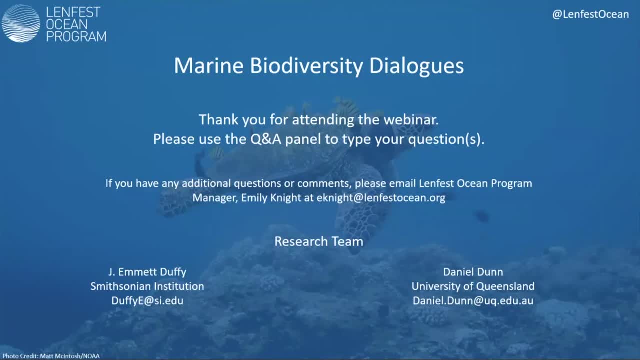 There are other projects ongoing. The work that NC says is not part of this project. There are other projects ongoing. We are working with LENFEST to map the footprint of human uses of the ocean. I think that are extremely relevant to this. 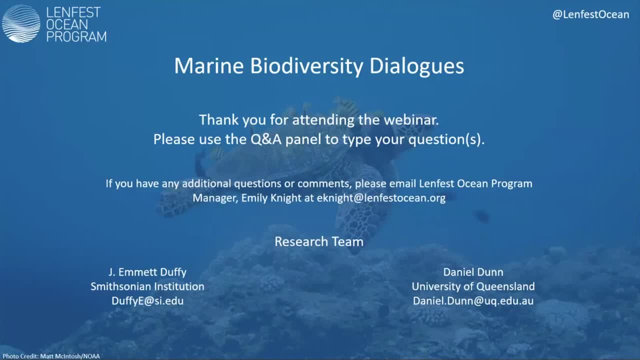 I think what we're trying very hard to do is to feed information on the biodiversity side that would then be incorporated down the line through more appropriate means of stakeholder engagements to decide how you want to put those together with human uses. next steps for the MPA network in the US. We are not going to do that. We are not trying. 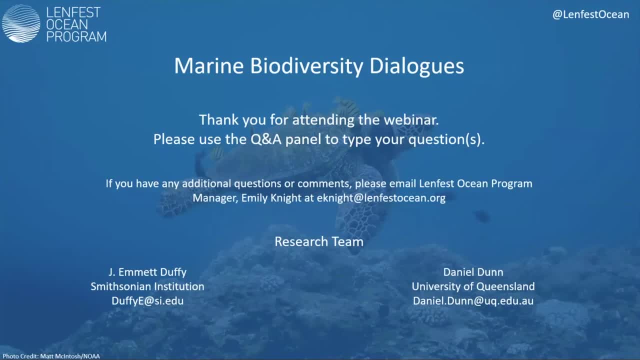 to determine which are the best places that you next need to choose. We're trying to identify gaps in the current coverage and then it will be up to, like I said, a more stakeholder-driven process to take a look at the threats and the costs related to those areas and determine. 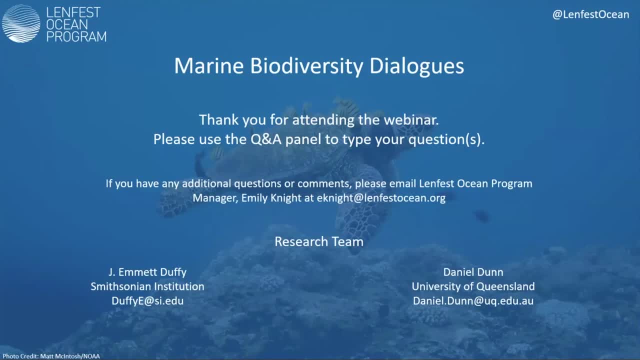 where they might want to go. Great Thank you. And we have one last question before we close out this evening, or morning or late afternoon, whenever you're joining: How will cultural heritage and its intersection with natural heritage be addressed in the GAP analysis, if at all? Will culturally? 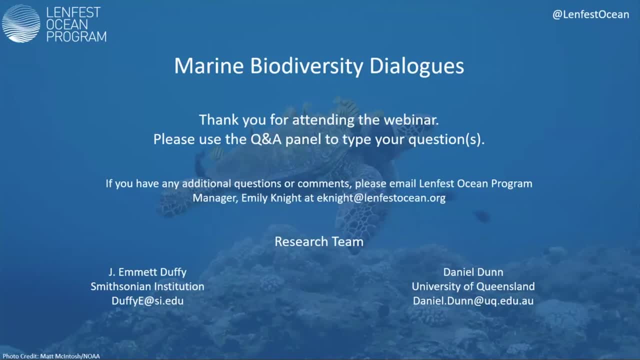 valuable species be prioritized for protection in any way? Okay, Yeah, that's a really interesting and important question and I think it, you know the answer is similar to Daniel's answer to the last question, which is, you know, the prioritization. 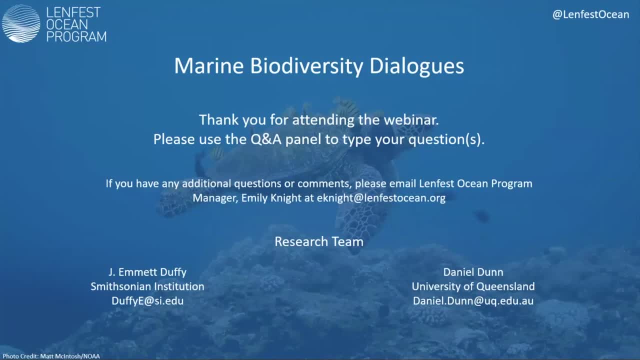 for conservation is again a stakeholder-driven process that you know is based on the values of the different stakeholders. You know our goal here is to show where the species are and are not protected and what kinds of… you know, habitats are protected and so on. So the way I would look at that is: I hope. 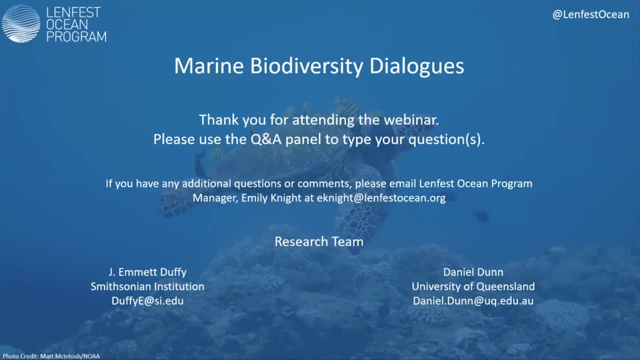 that the products of this work make it possible to more effectively protect cultural heritage in an evidence-based way- Great. Thank you so much, Daniel. do you have anything to add before I wrap it up? No, just a huge thank you to everybody for joining and for staying on to the end here.